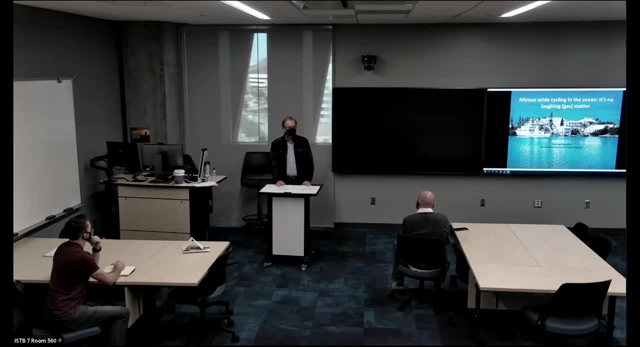 from the ocean into the atmosphere, And these gas exchange measurements are pretty tricky to do. He's using the Eddy covariance method. that reminded me of my work, where we actually released two tracers and watched how they came back out into the atmosphere. Whichever way you do it, that's a. that's a. 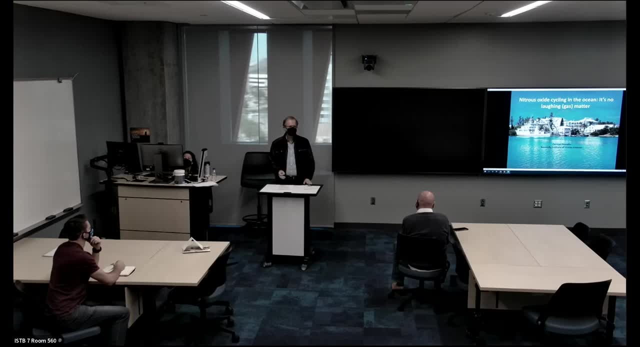 tricky measurement, So I think he told me he's still making his way into that, but it's a very interesting facet of his work. Before joining BIOS, the Bermuda Institute of Ocean Sciences, Damian was a postdoctoral scholar and research scientist at GEOMAR, which is a research center for marine science in 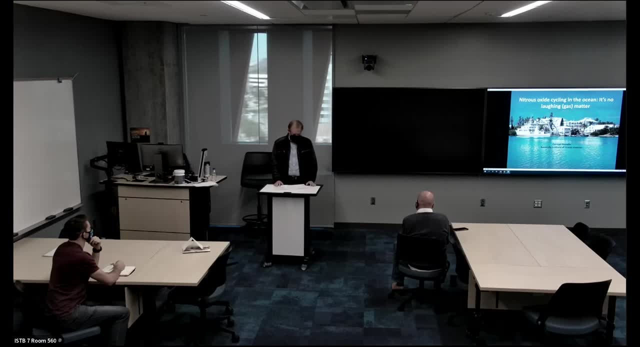 Kiel, Germany, And he got his education in his PhD In biogeochemical oceanography at the University of Victoria, Canada, in 2012.. So, without further ado, I'd like to hand over to Damian. Thanks, Peter. 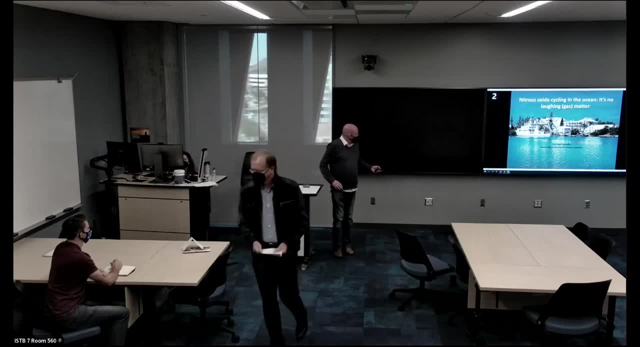 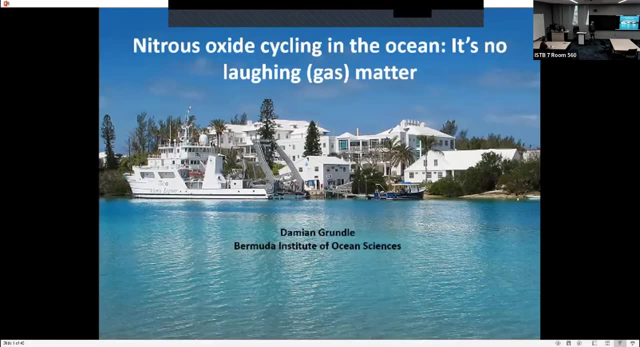 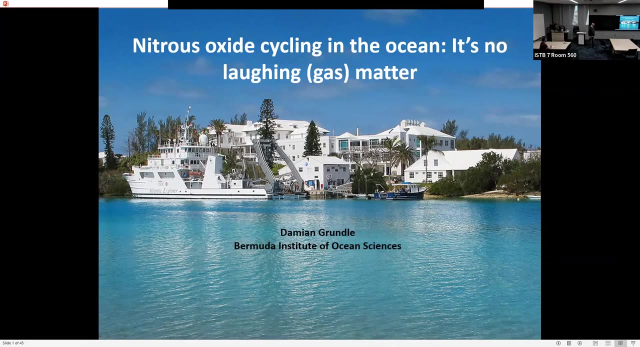 Thanks for everyone for coming along today and thanks for inviting us out here this week. It's been an enjoyable morning and looking forward to more chats And tours around campus as the week goes on. So, as Peter mentioned, I'm going to talk about nitrous oxide cycling in the ocean. 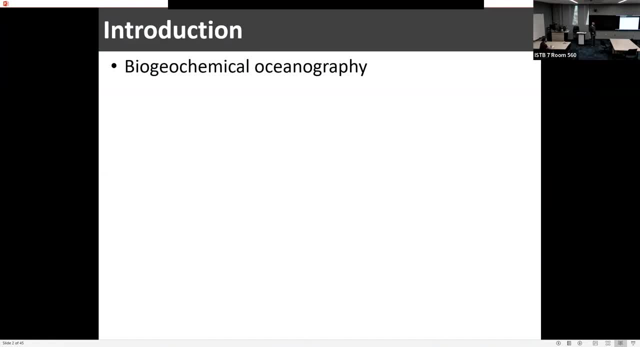 First off, just as Peter mentioned a little intro, I'm a biogeochemical oceanographer. This- principally from my side of things at least, includes sort of the study of the interaction between biology and chemistry in the ocean. One of the primary things that I really focus on is the marine nitrogen cycle. 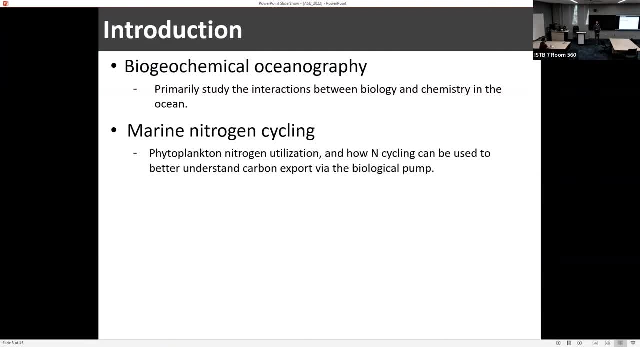 And this is a whole suite of things, So it includes things like looking at phytoplankton nutrient utilization in the ocean And how end cycling can be used to better understand carbon export via the biological pump. Right now we're actually I have an NSF funded project where we're using, with my co-PI's Ruth Curry and Mike Lomas- 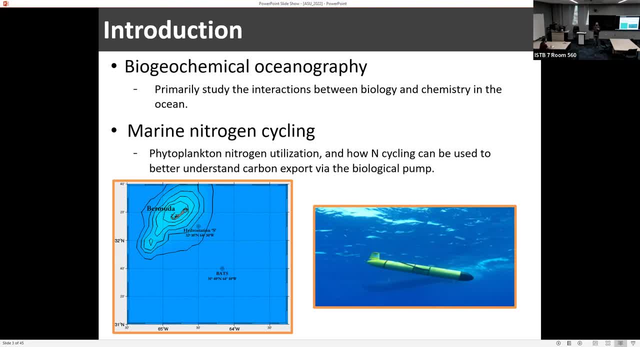 we're using gliders to equip with a whole bunch of sensors, including nitrate sensors and micro turbulent sensors, to be able to sort of detect the upward movement of nitrate into the euphotic zone and better- oh, excuse me, better- understand that. 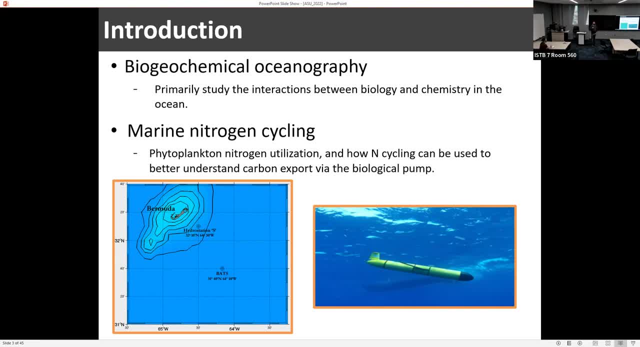 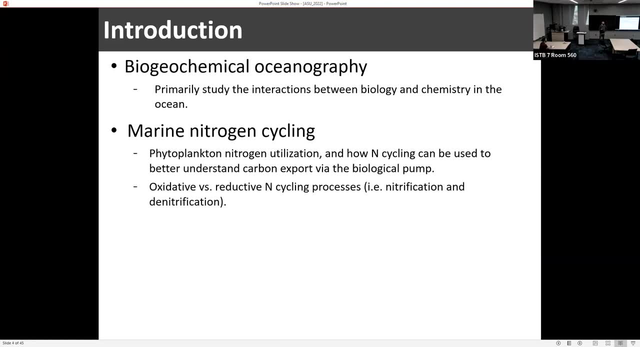 Export production at much higher temporal resolutions than we could achieve by just simply going out once a month on a ship. I also look at oxidative versus reductive end cycling pathways. So this includes nitrification, which is the biological oxidation of ammonium to nitrate. 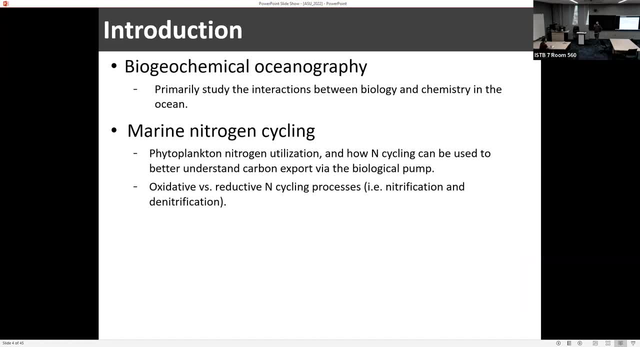 And then denitrification, a reductive pathway which looks at the reduction of nitrate to N2 gas and leads to a loss of bioavailable nitrogen from the ocean. I mentioned what I one of the main things I look at is also nitrous oxide cycling in the context of nitrification and denitrification. 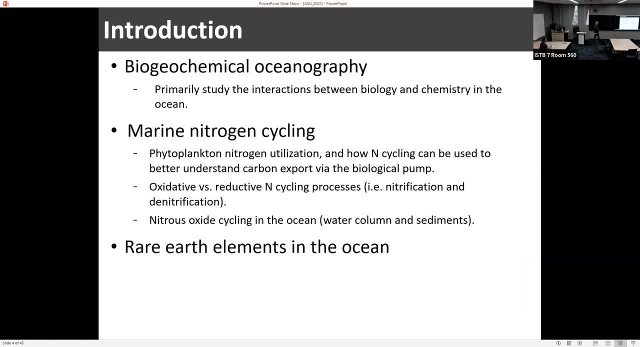 And I'll come back to this in a second. Much more recently I've also with an amazing student that I have worked with me, Annelies Meyer, who's now in the MIT HUI PhD program. We were looking at rare earth elements in the ocean in relationship to methane cycling. 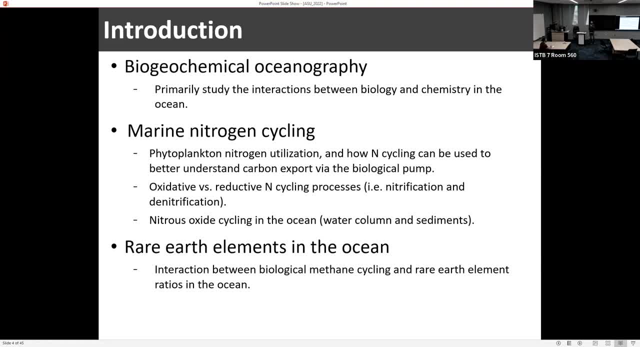 And we recently just published a paper, And we recently just published what I thought was a pretty cool paper- I'm still learning a lot about this from Annelies, But recently just published this in Earth Planetary Science Letters And we're able to look at rare earth element ratios to sort of understand what's been going on with methane in the ocean. 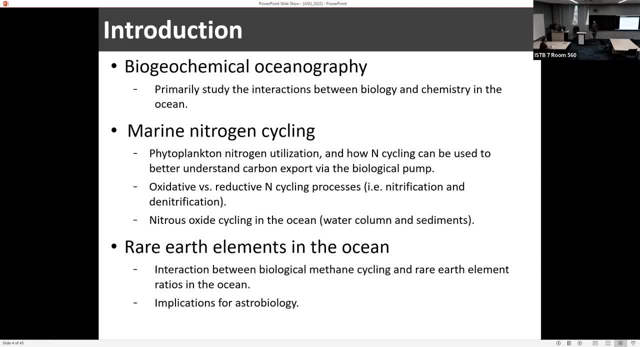 But it also has some pretty cool sort of potential implications for things like astrobiology. Imagine if we can go off to a planet, let's say Mars, where we detected methane. We can bring back soil samples and look at the rare earth element ratios. 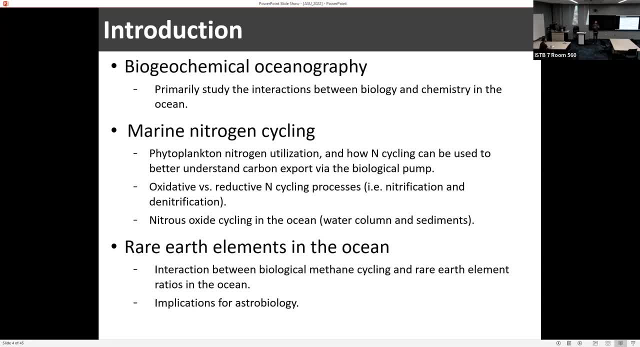 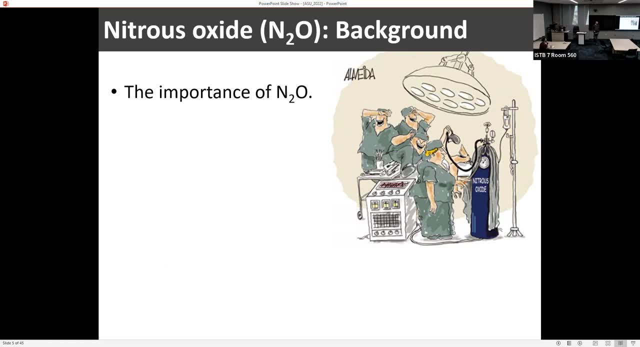 And we might be able to start saying something about whether this was due to biological activity or not. As I said, the main focus of today is nitrous oxide seismic, So I'm going to start off with just touching on the importance of N2O. 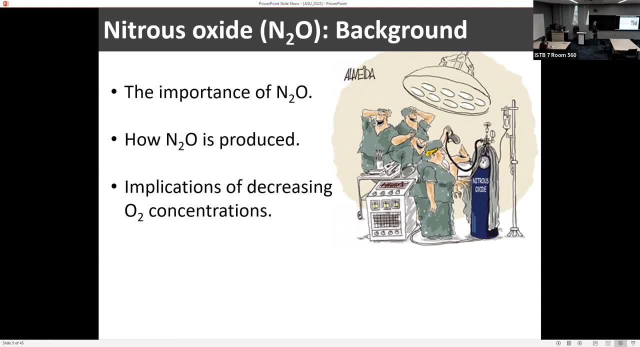 How N2O is produced, The implications of decreasing oxygen for N2O production in the ocean. Give you some examples of past and more current sort of research activities And then touch on some of those. And then touch on some thoughts I have about future research. 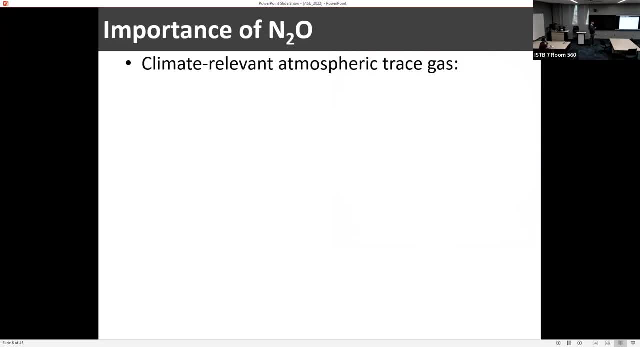 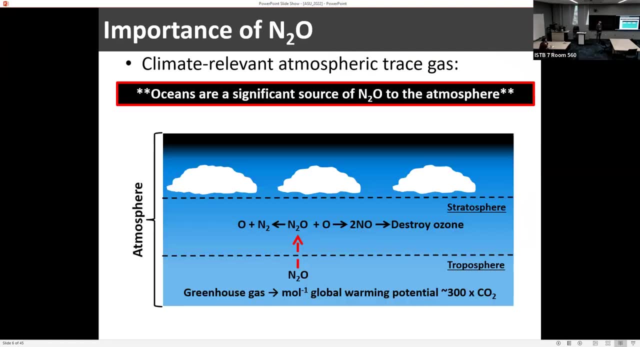 So, first off, N2O is a climate relevant atmospheric trace gas, And the oceans are a significant source of N2O to the atmosphere. We take a look at this schematic here. What we see is when N2O is well, when it's produced in the ocean, it's eventually ventilated to the atmosphere. 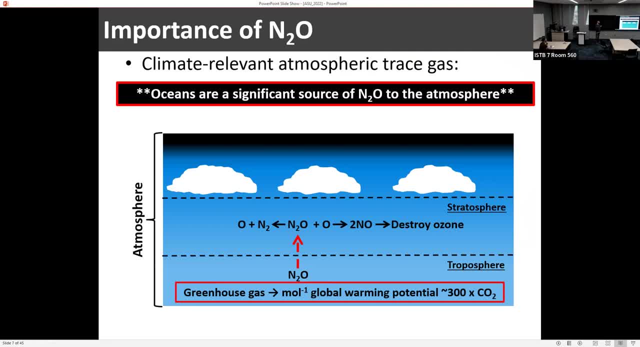 When it first enters the troposphere, And here it acts as a greenhouse gas With a per mole global warming potential Which is about 300 times out of carbon dioxide. After some period of time that N2O will survive transport up into the stratosphere. 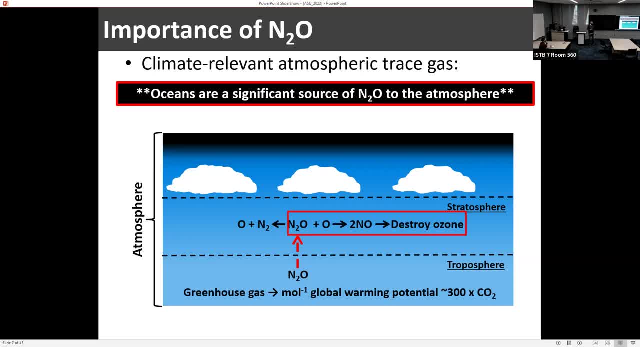 Where it can undergo reactions that destroy ozone. So we've got a gas that's having a two prong effect here in the atmosphere, On one hand contributing to atmospheric warming, On the other hand it's contributing to ozone destruction And, since the Montreal protocols and the reduction of CFCs, 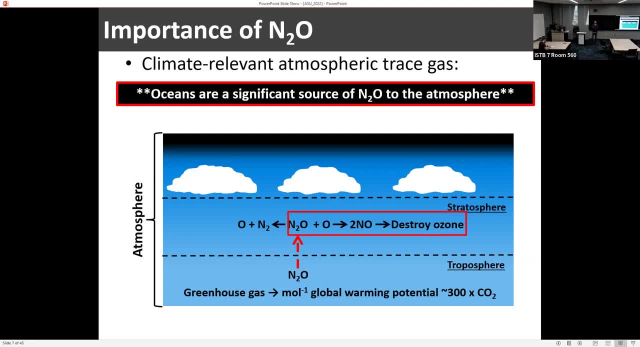 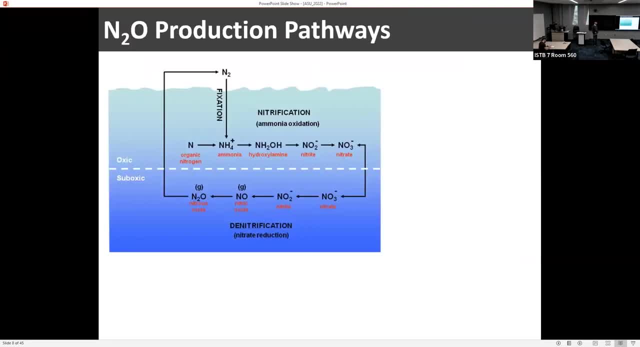 N2O has been identified as being a greenhouse gas. It's been sort of the number one ozone destroying gas as we move through this century. So now, just briefly, the production pathway. So here we've got these two major sort of end cycling processes that I mentioned before. 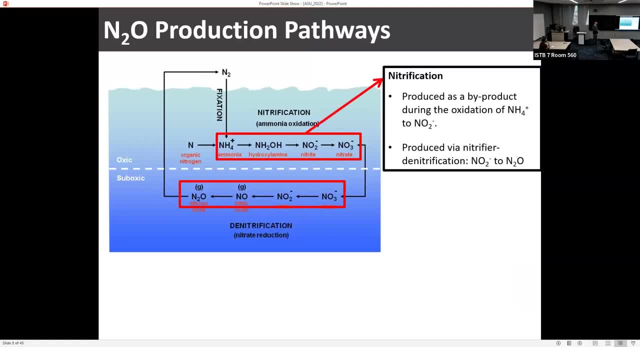 Nitrification and denitrification. In nitrification, N2O can be produced as a byproduct. during the oxidation of ammonium to nitrite, The first step of nitrification, Those same nitrifying bugs can also reduce under certain conditions. 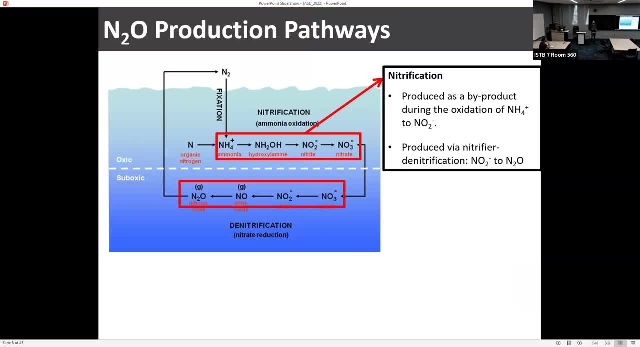 Can reduce nitrite to N2O through what we call nitrifier denitrification. In the more canonical or canonical denitrification, N2O is an intermediate in the reduction of nitrate to dinitrogen gas, So it's being both produced and consumed. 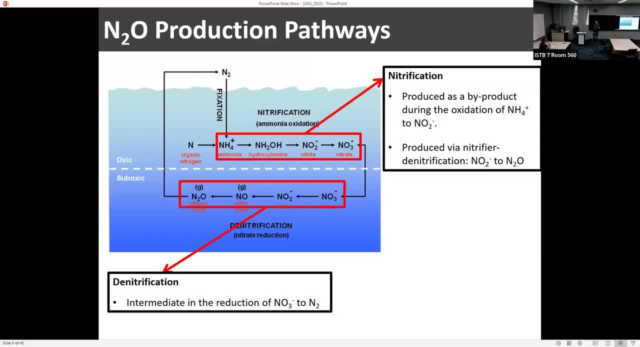 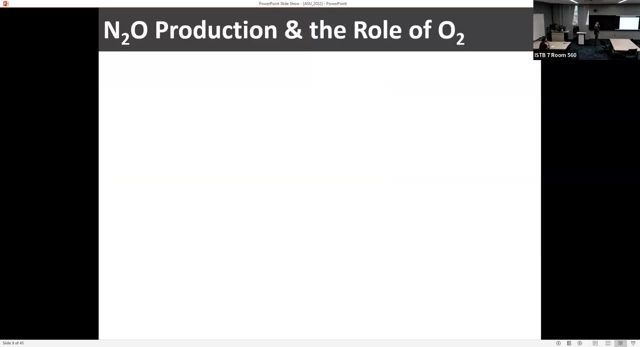 But under the right conditions, Denitrification can produce more N2O than it consumes, So it can be a net producer of N2O. Looking right now at the sort of theoretical role of oxygen in the oceans on N2O production, 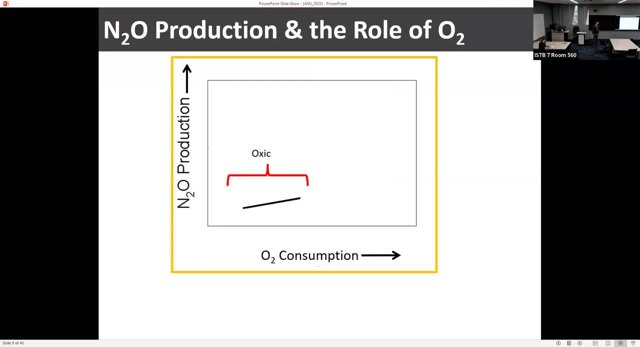 So we've got N2O production on the y-axis, Oxygen consumption on the x-axis, When we have fairly oxygenated conditions in the ocean, The amount of N2O produced versus the amount of oxygen consumed, Which is an indicator, let's say, for how much nitrification has been occurring. 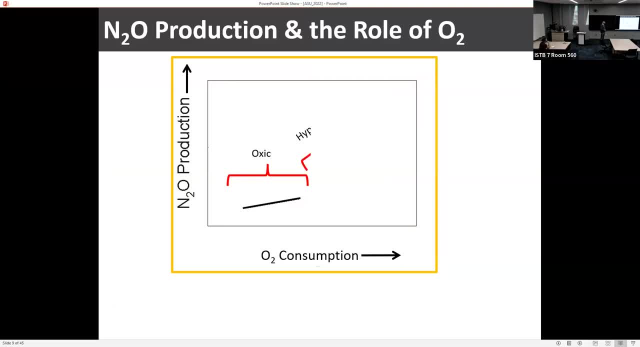 We see very low amounts of N2O being produced, But as we get into low oxygen conditions That N2O production can really increase, Or the amount of the number of moles of N2O produced for every mole of oxygen consumed increases. 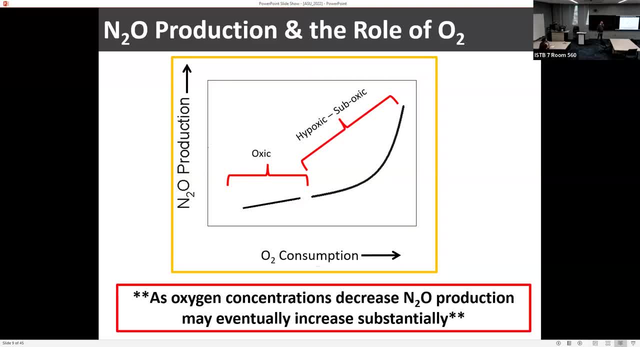 Really, the take home message for this is simply that oxygen concentrations decrease At some point. N2O production could eventually start to increase quite substantially, And this raises some cause for concern Because, as I'm sure many of you are aware, Oxygen concentrations in some regions of the ocean are decreasing. 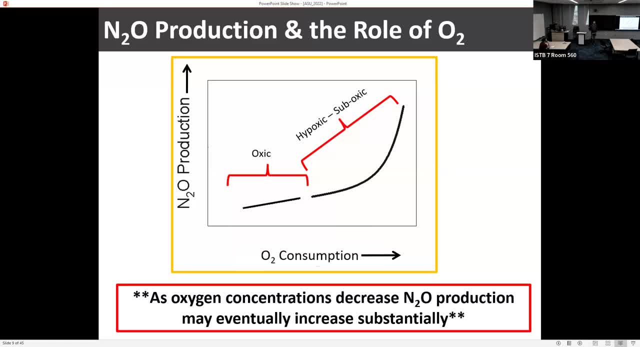 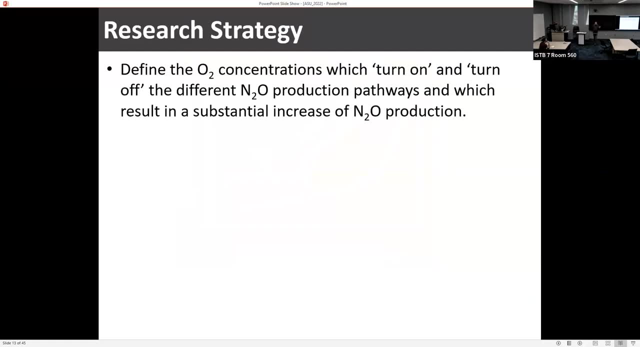 Oxygen minimum or oxygen deficient zones are increasing in size And the frequency and the intensity of coastal hypoxic events is increasing. So at some point through the century it's likely that we're going to see N2O production really ramping up. So this is what a number of years ago, when I started getting interested in N2O- 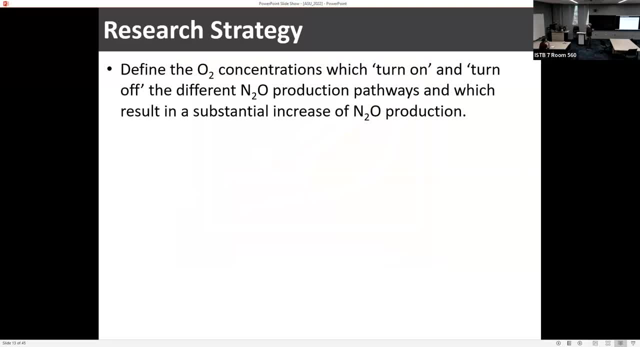 And I wanted to sort of set up my research strategy. I defined it as being: I wanted to set my research strategy to essentially define the oxygen concentrations Which turn on and turn off the different production pathways, And the oxygen concentrations are thresholds which lead to large increases in N2O production. 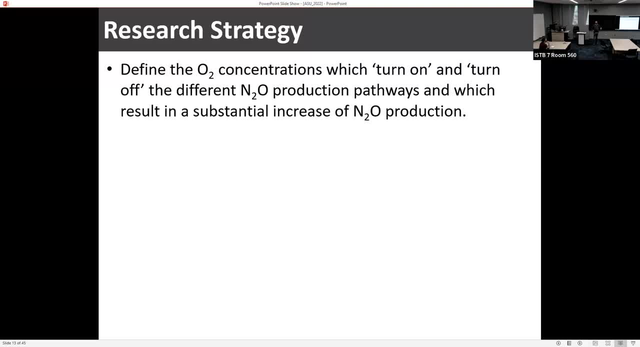 If we can start to do this, Then we can start to predict at what point through this century will N2O production really increase, And by how much it will increase, And then how much will be released to the atmosphere. So the next sort of question to address is: 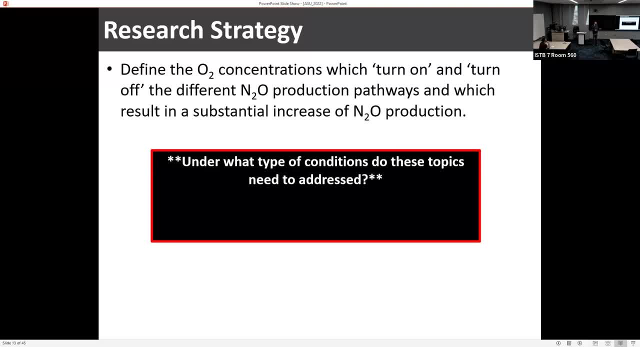 Okay, Under what kind of conditions do we want to address these topics, And by that I just simply mean: do we want to do this in the lab, Or do we want to go out in the field and look at this in real world conditions? 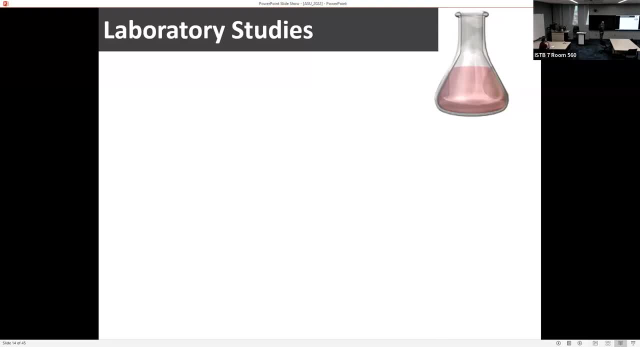 So, as far as lab studies go, There have been a number of very important lab studies that have given us some real insights into the role of oxygen and N2O production. The first was- And I'm just going to touch on a few here- 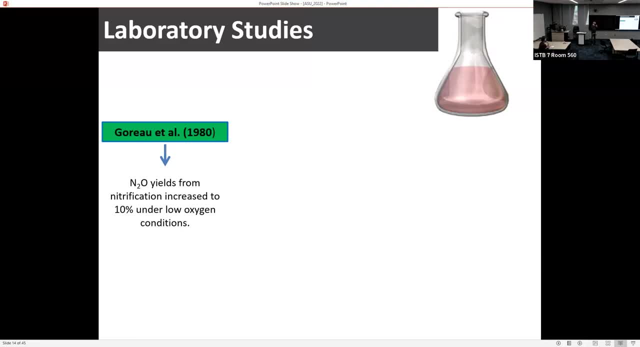 So the first was- This was the first sort of real major one- Goro et al 1980. And they cultured ammonium oxidizing bacteria. What they found was that as oxygen concentrations decreased and got very low, N2O yields increased in about 0.03% to 10%. 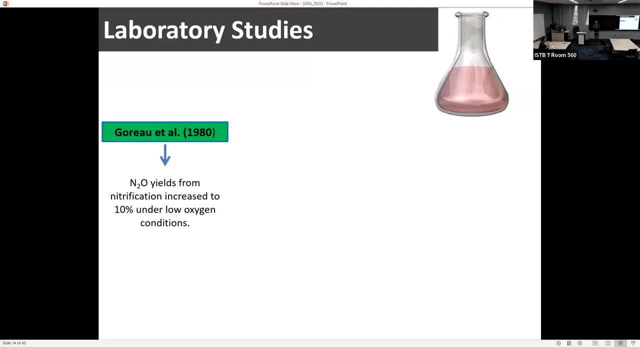 When I say yields or percent yield, I'm going to be interchanging N2O production and yields. Yields: I'm just referring to what percentage of every mole of ammonium is oxidized Has been yielded as N2O. So this was a massive increase. 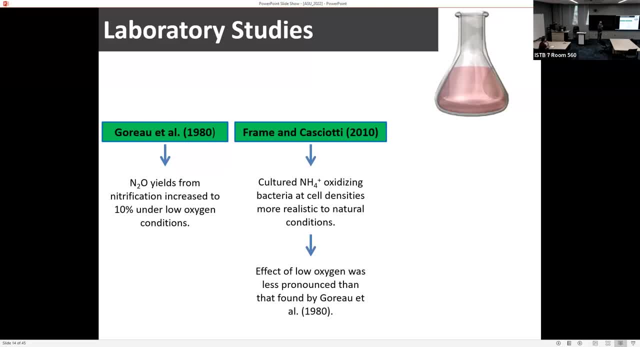 About three decades later, Freeman Casciotti came along And they cultured ammonium, oxidizing bacteria Concentrations, Or sorry, Cell densities, More realistic natural conditions, And they found that, Yes, Okay, N2O production does increase. 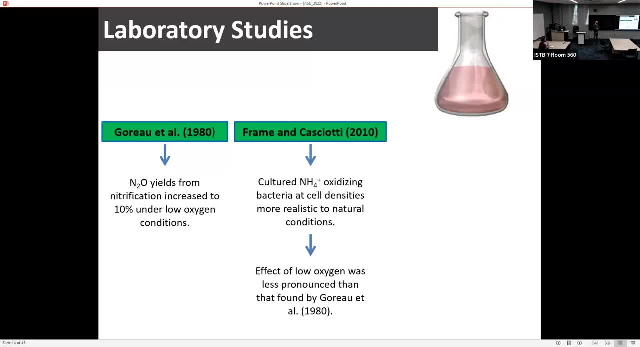 But the effect wasn't as pronounced as the Goro et al study. However, Alison Santoro then showed that It's actually the ammonium oxidizing bacteria that are capable of producing Much more N2O than their bacterial counterparts under low oxygen conditions. 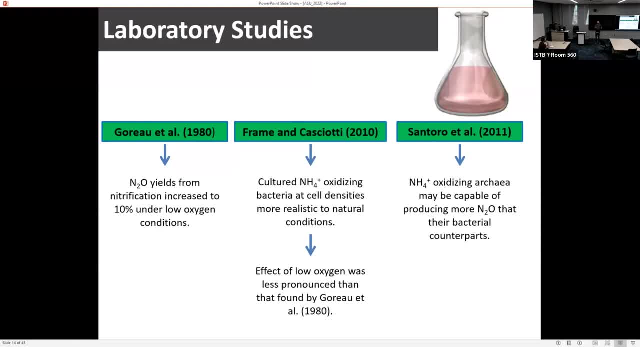 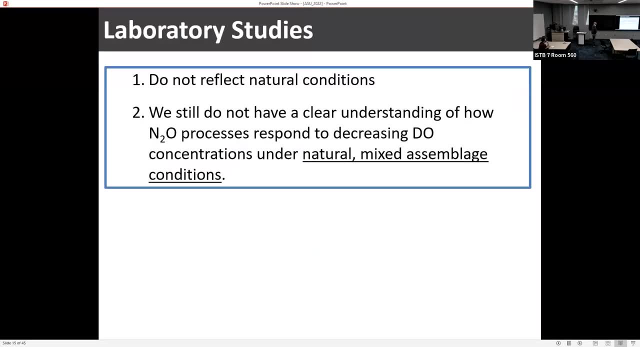 So again this brings us back to if we're in a, You know, in the field With mixed assemblages, We're likely to see an increase in N2O production Under low oxygen conditions. Those lab studies have given us some really important insights, but 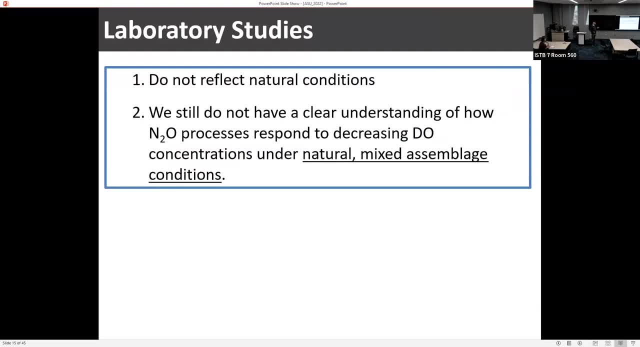 You know, the fact is they don't reflect natural conditions And at the time- I was sort of getting into this, I would say we still, You know, we didn't have a clear understanding of how N2O processes Would respond to a decrease in dissolved oxygen concentrations. 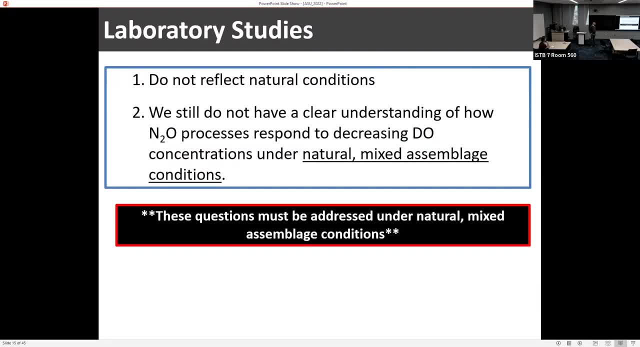 In under natural conditions. So, basically, I pointed out that then we really need to start addressing these questions under natural mixed assemblage conditions in the field. So we need to go out to sea and do this, Having decided that the next thing was okay. where are we going to do this? 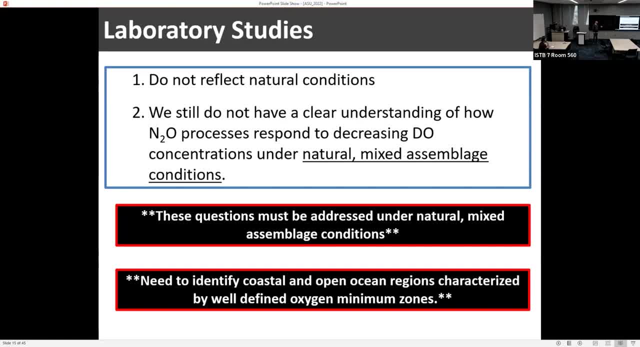 Work, You know. to do it, we really then need to identify coastal and open ocean regions that are characterized by Well-defined option minimum or option deficient zones. Put another way, You know, steep option gradients Where we're going from oxygenated surface waters. 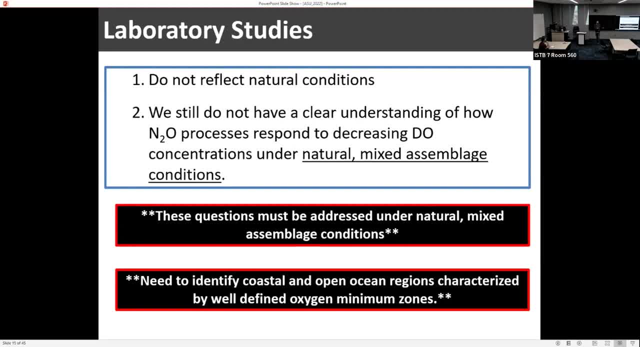 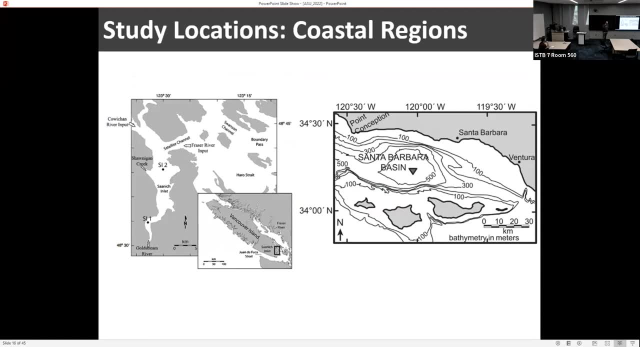 Down to very low option, even anoxic, zero auction conditions At more intermediate deaths. So we're basically using these systems as natural laboratories, Just to give you some ideas about some of the reasons we've worked in, And actually I'm going to use this as sort of segue into something I wanted to sort of 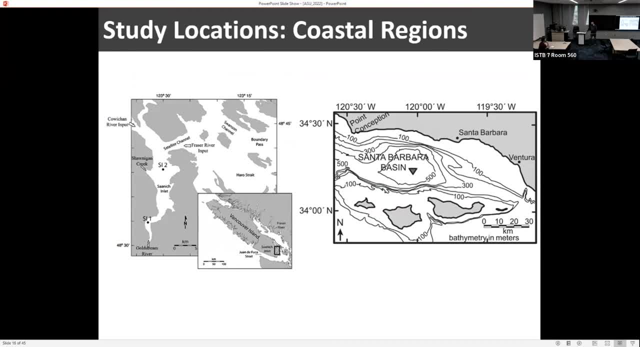 highlight- And that is Something I wanted to sort of highlight as well, And I think Nick mentioned this briefly last week- is that, Well, a lot of us said, well, all of us at bias, we do have a research footprint. 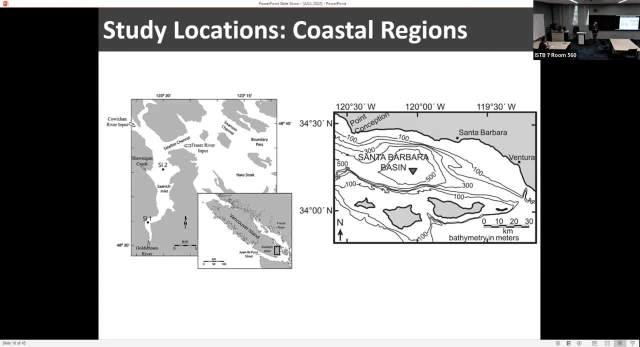 In the Sargasso sea and the waters around Bermuda. But a lot of us also work all over that The globe, you know, in the Pacific and the Atlantic and coastal regions and so forth, And this was sort of highlight this little year. So 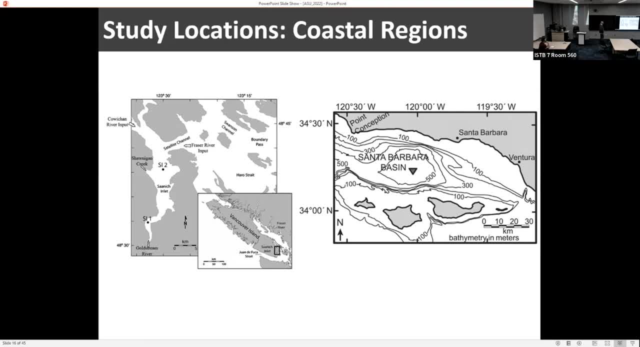 A couple of you know some of the coastal regions that we worked in Well. Santa Jean led on Southern Vancouver Island. I've worked in this region a lot. It's a great natural laboratory for Sort of understanding the impacts of auction. 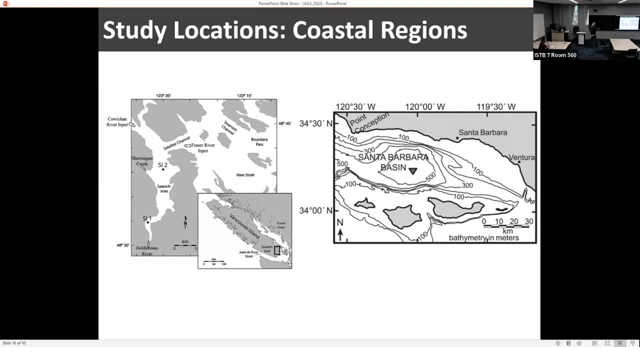 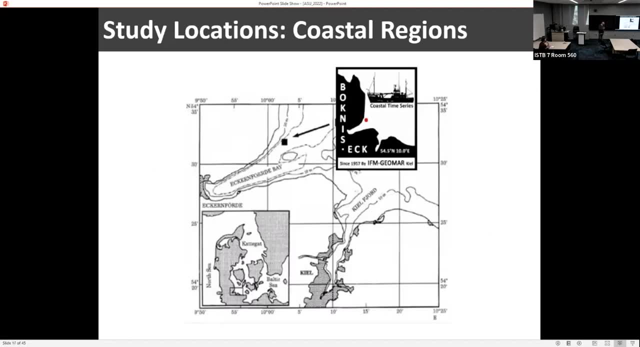 On biogeochemical processes. We've published work from the Santa Barbara basin using a cow coffee time series Data Also worked in a bottom sec, which is a time series station Around by Herman In the Baltic sea just in. 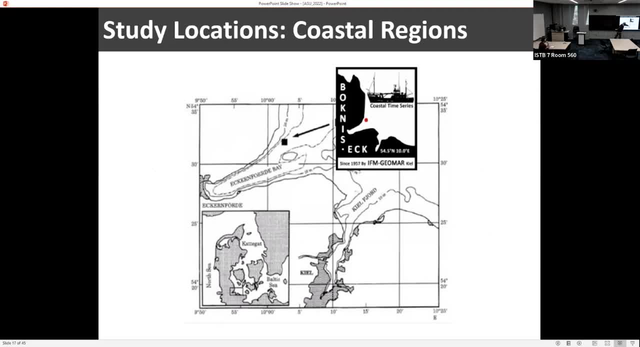 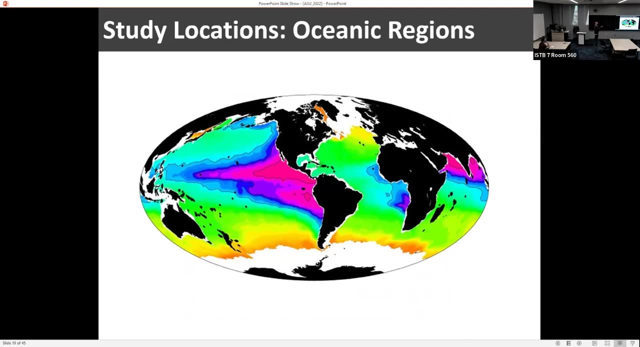 Bay here. So Institute is here. Just go out Around the corner And collect samples. And about the? what about the open ocean? So This figure shows auction concentrations At intermediate deaths around the globe. Well, it's ocean, Sorry. 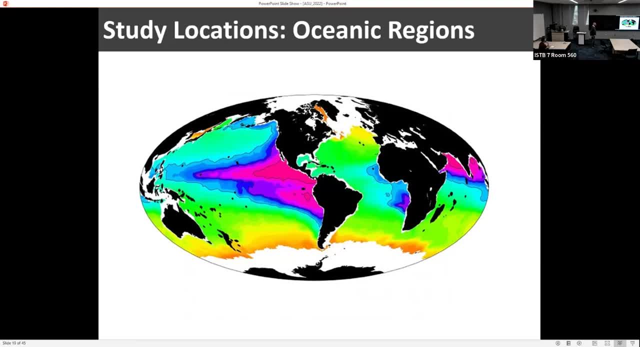 I'm going to apologize, but the the scale Hasn't popped up there, But essentially the Part of the pink, The lower the option concentration. So we've got a couple of major zones, We've got the Eastern tropical north. 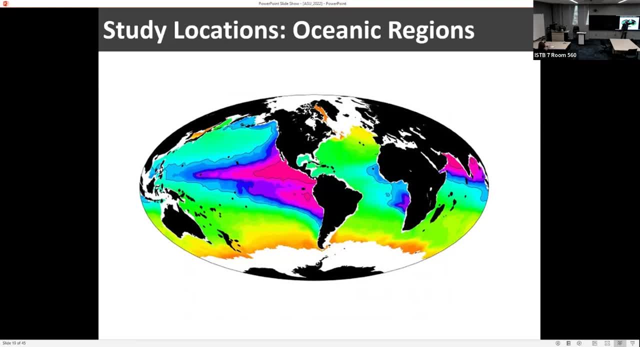 And South Pacific, And then we've got the Indian ocean, Something here going on here in the Benguela Upwelling system, But the auction concentrations still don't get very low As far as In the context of nitrogen cycling. 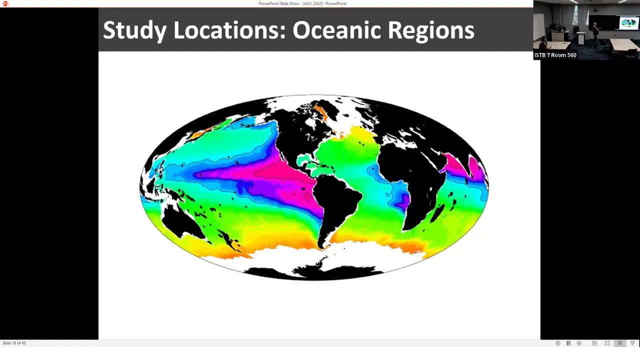 We're not going to see any major changes, And that's true Pretty much of the entire The option. There's an exception to this, which I'm going to touch on In a few slides time, But Let's now move on to. 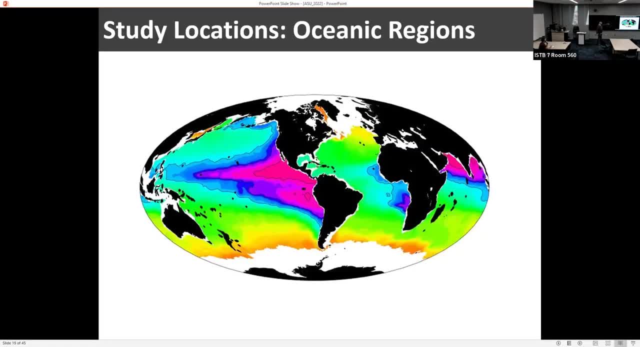 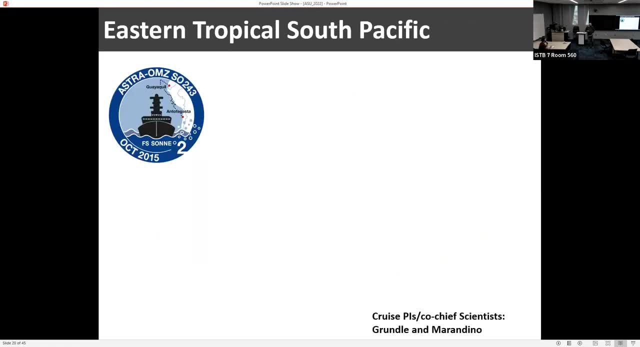 Oh sorry, So yeah, just to give you an example, then, Of one of the you know the cruises we've operated in these regions, So in 2015.. Myself and my co-PI and co-chief scientists. 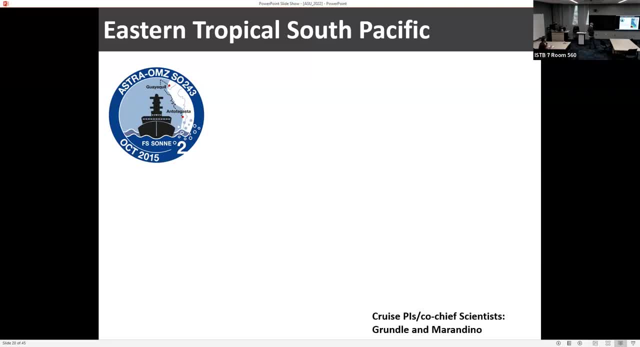 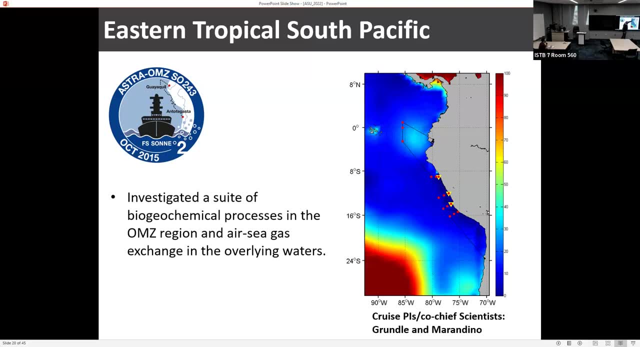 Krista Marandino around the The Astro OMZ cruise. So here we've got Just a figure showing the Track. So north went north of the equator And drop down through Peru Or in the waters of Peru, And then we've got. 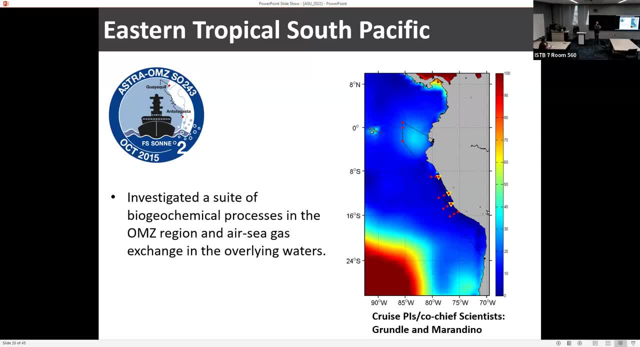 And then we've got the Pacific coast At the bottom of the equator, And then we've got A little bit of the Pacific coast, Terminating and chilling. In this case, I apologize- The scales now flip. So now the darker, the blue, the lower, the auction. 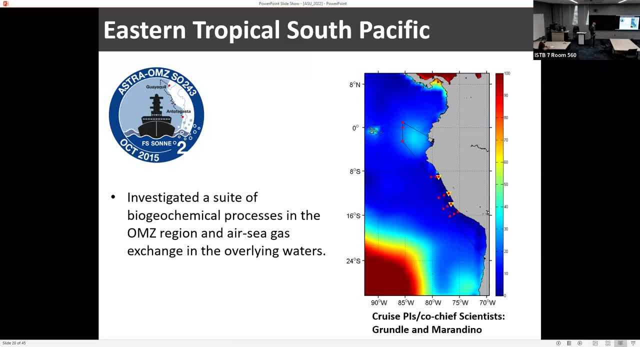 Concentration. So we had funding to support about 36 scientists or PIs and technicians On this cruise And that we investigated a whole suite of biogeochemical processes And the option minimum region, As well as The gas exchange and the overlying surface. 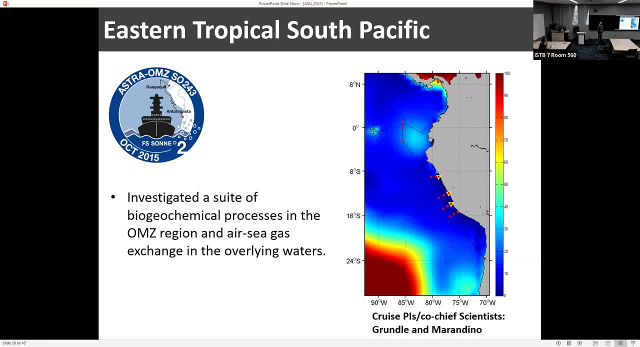 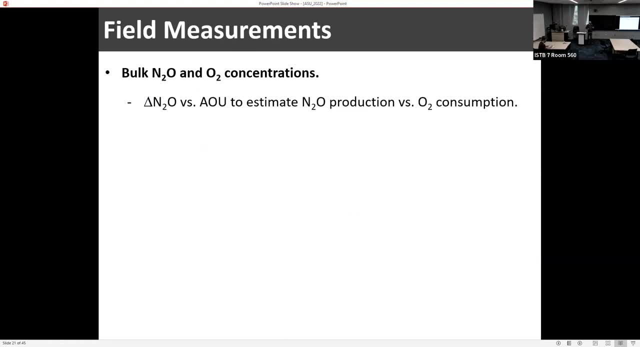 Waters. Obviously, One of the main focuses From my group was the nitrous oxide store story. So those are some of the regions we work in. Now what about the kind of measurements we make and how do we interpret? how do we use these to sort of understand N2O cycle? 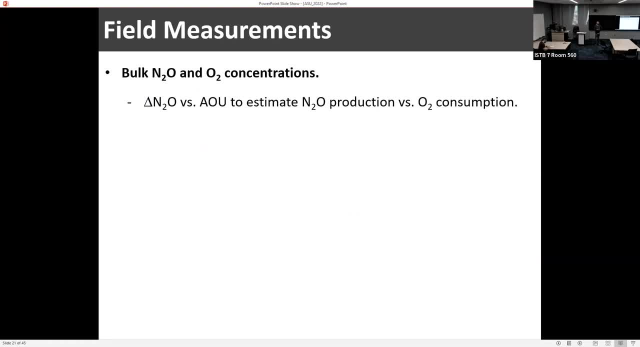 So first off, very straightforward, we need N2O concentrations and oxygen concentrations. From this we can calculate things like del N2O and AOU. Del N2O is essentially a measure of how much, or an estimate of how much N2O has been produced- excuse me, within a parcel of water. 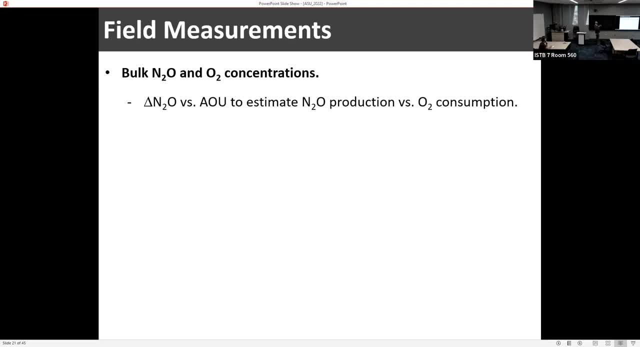 since it was last in contact with the atmosphere, So we can think of it as N2O production, or how much has N2O been produced? AOU, or apparent oxygen utilization, is an estimate of how much oxygen has been consumed within that same parcel of water since it was last in contact with the. 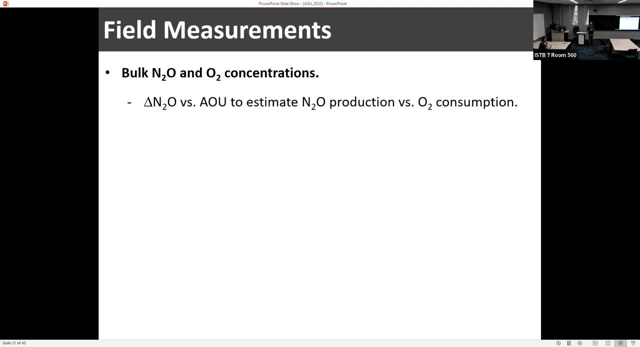 atmosphere. So we can look at this now as sort of N2O production versus oxygen consumption. Let's give you an example. This is some data from the eastern tropical south Pacific. So we've got del N2O on the y-axis, AOU on the x-axis. What we see is that as oxygen, 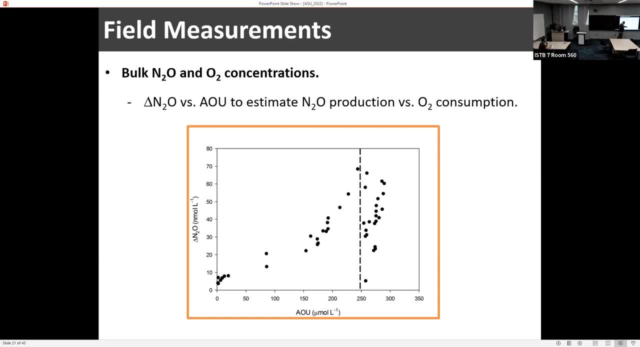 concentrations decrease or, as oxygen consumption increases, the amount of N2O being produced versus the amount of oxygen being consumed increases. That is until we get on the right side of this dashed line And that represents the anoxic zone, so where we've got no oxygen present at all. 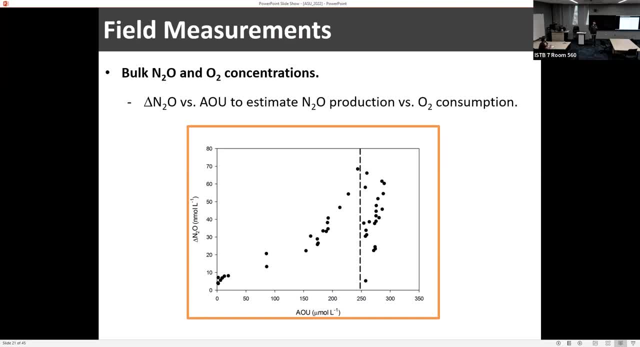 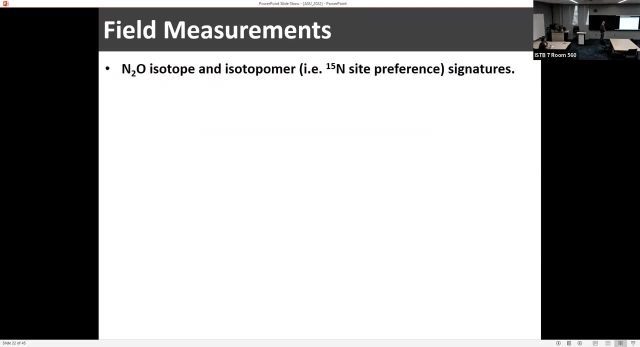 And denitrification is switching from being potentially in that source to now being in that sink, So it's starting to consume N2O and remove it from the water or convert it to dinitrogen gas. We then also use N2O isotope and isotope signature measurements. So 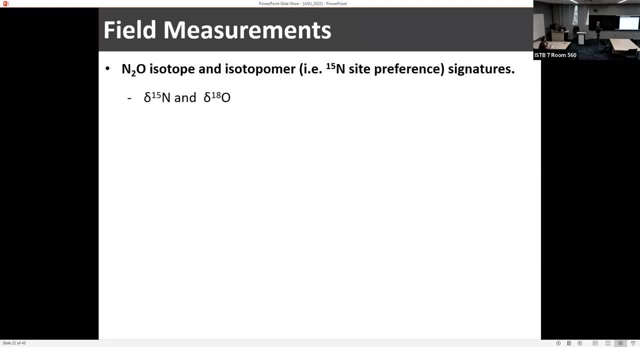 by this I mean looking at the del 15N and del 18O signature of N2O And then the 15N site preference, which is the intermolecular distribution of 15N in that linear NNO molecule. We can use these measurements to start to identify. 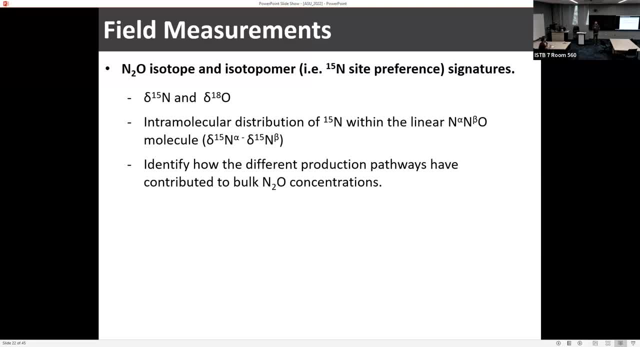 how the different production or cycling pathways have contributed to the bulk N2O concentrations that we see in the water, So we can understand which processes are really contributing to the N2O that we're seeing in the ocean and then that's getting to the atmosphere. 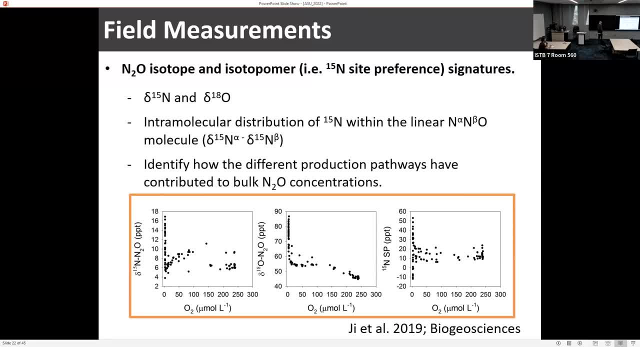 as well. So just to give you an example, this is data from a paper that my postdoc- or just previous postdoc- and I recently published in Biogeosciences, And this is: we've got the del 15N of N2O on the left, the del 18O in the middle and the 15N site preference on the right. 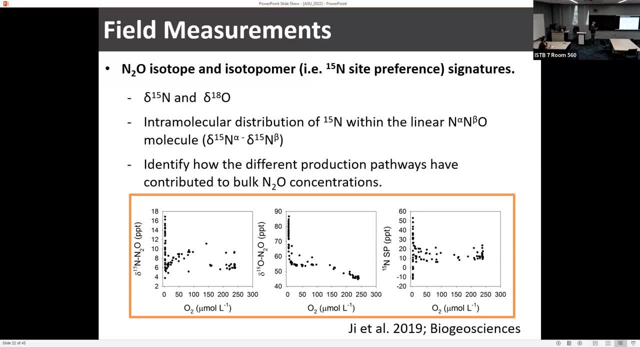 I'm not going to go into detail about this, but I just want to sort of highlight that you can see, as we get down and oxygen concentrations decrease, at some point the signature, the isotope signatures, really shift. So we can start to pry apart and understand, okay, what point. 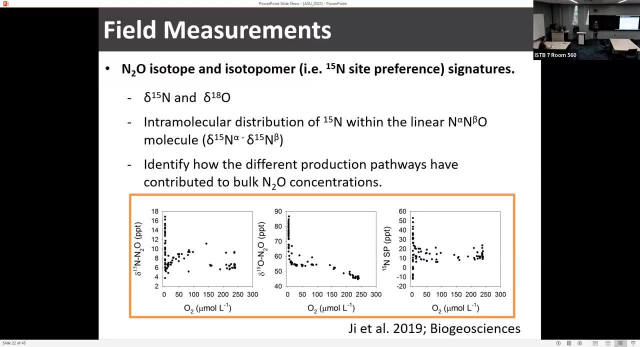 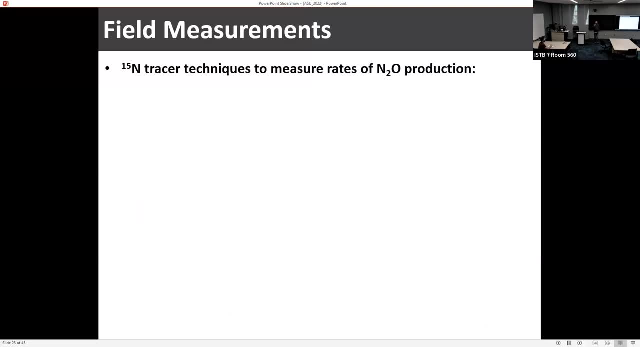 do the nitrifying bugs start switching onto nitrify or denitrification? At what point does nitrification start being a net producer of N2O and at what point does it start to consume N2O And use 15N tracer techniques to measure the actual rates of N2O production at the time we're 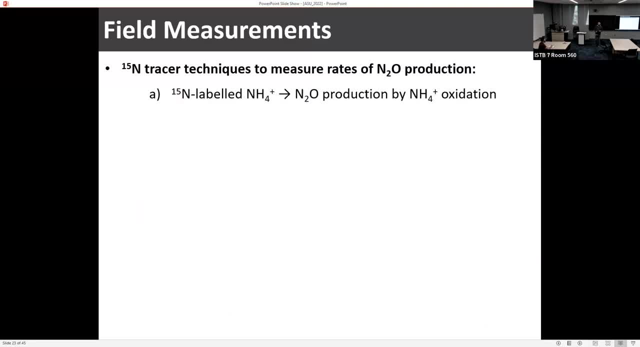 sampling. So we can take a sample of water in a gas-type vial, let's say from a Niskin bottle on a ship. We can inject it with 15N-labeled ammonium. We can trace that 15N from the. 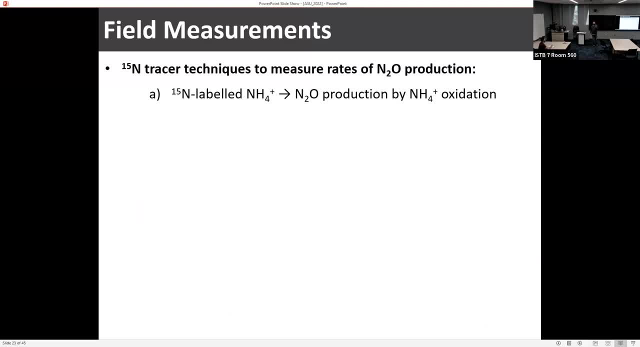 substrate, pool, the ammonium pool into the N2O And actually calculate the actual rate of production. We can do that under varying oxygen concentrations. You can also do this with 15N-labeled nitrite and 15N-labeled nitrate to. 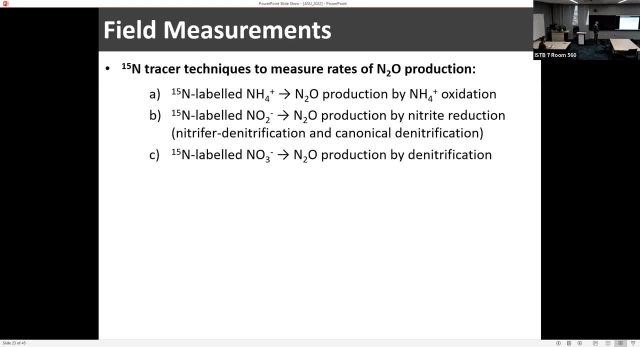 look at N2O production from the reductive pathways. I'll just give you an example here. So this is from a paper that my postdoc, Jimmy, and I also just well, a couple years ago, published in the Journal of Geophysical Research. This is from Sanagin Lab And we've got nitrification yields. 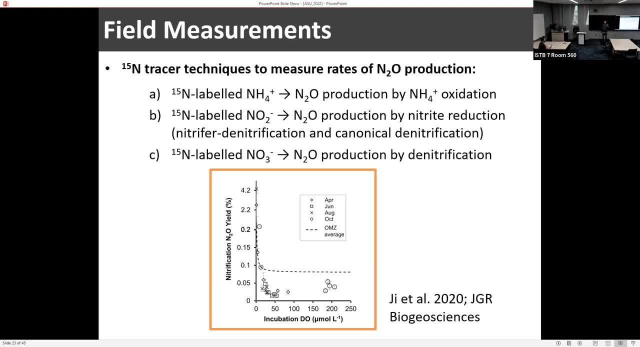 Remember, this is the percent of ammonium that's turned into N2O. This oxidizer ends up turning into N2O. We've got nitrification yields here. We've got the oxygen concentration during the incubation period on the x-axis. You can see that, the yields when we've got you know. 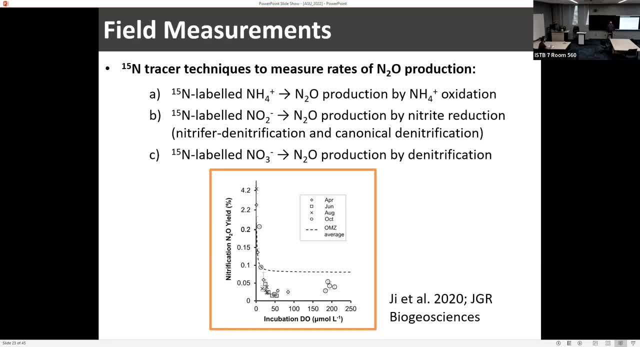 oxygen concentrations going down to about 20 micromoles per liter. the yields are pretty low. We're talking, you know, around, about, let's say, 0.05%, But as soon as we drop below about 20 micromoles per liter, the N2O yields skyrocket. We're getting 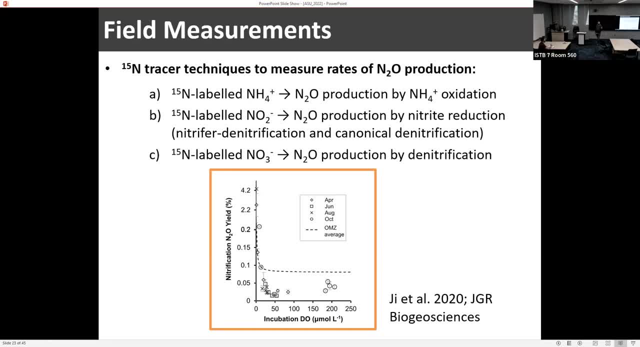 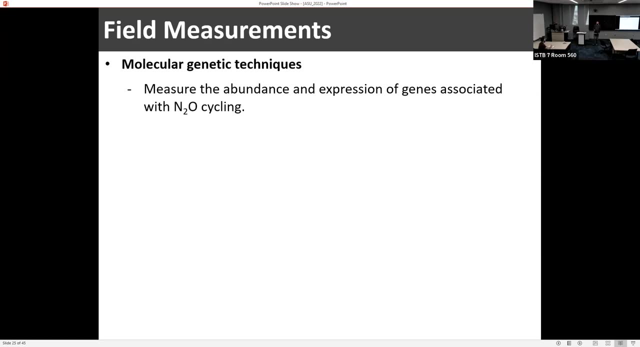 up to, sort of now, about 4% yield. So this is again sort of just demonstrating that you know the kind of oxygen thresholds where we see these large increases in N2O production. And finally, I don't make these measurements myself, but through collaborations. 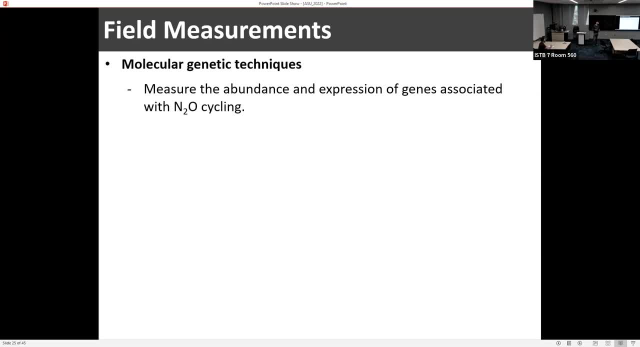 we also look at the abundance and the expression of genes associated with that, with N2O cycling. So when are these turning on and turning off? And then, finally, I use microsensor measurements from microelectrodes to look at investigate N2O cycling in marine sediments. 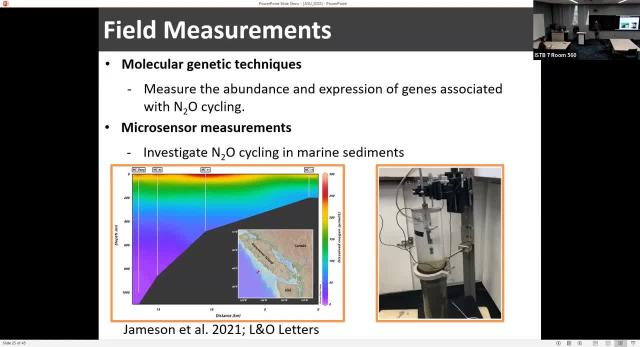 And I'm working largely with, so I'm an adjunct member of the Faculty of Graduate Studies at the University of Victoria. One of the students I'm co-advising, Brett Jamieson, has been using my lab to look at N2O cycling in marine sediments, And this is just an example of one of the projects. 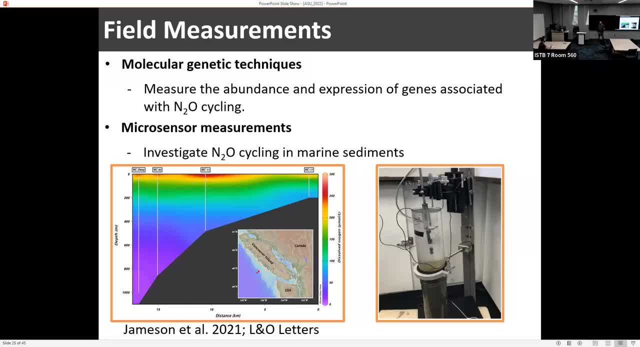 we ran. This is in the continental margin off of Vancouver Island. So we went out on the ship with a submersible, We went down and we collected sediment cores at various depths. We brought those cores back up to the surface. It was an autonomous vehicle. We weren't actually physically in it. 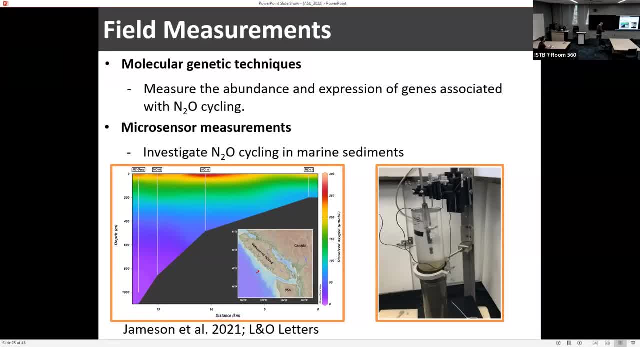 And we incubated those sediments in chambers. We're flowing seawater for periods of time And every so often we can take those cores out and we take a microsensor, which is a very minimally invasive approach. I don't know if you can see it very well here. It's. 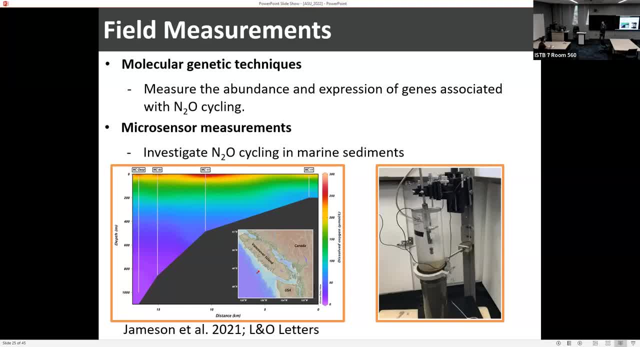 a very fine sort of needle. It goes through the sediment core, very high resolution, vertical resolution, And we can measure N2O concentrations and oxygen concentrations. We can then apply curve fit modeling techniques to those results And we can estimate how much. 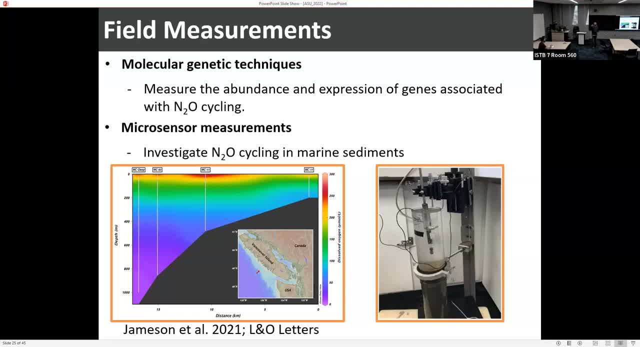 N2O is being produced, how much is being consumed, how much is getting out from the sediments to the water or vice versa? And in this case we found that the sediments were a very important source of N2O to the water column. 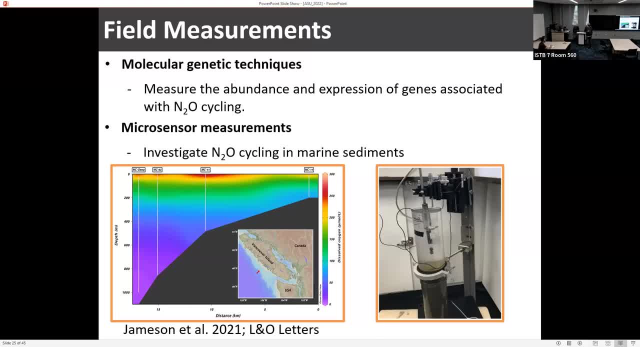 We're just wrapping up another paper where we did this in twisting mangrove sediments around Bermuda And in that case we found that those sediments are really important sinks of N2O. So they're drawing N2O out of the water column, which provides another argument for let's leave these. 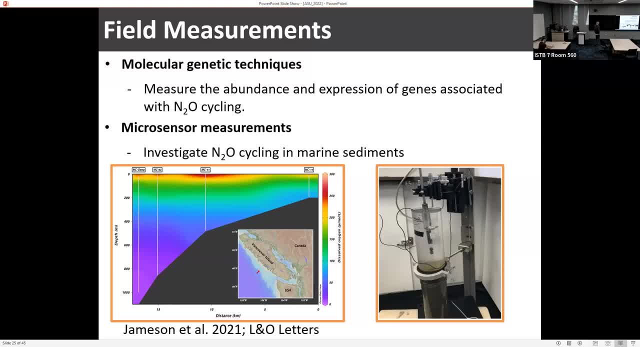 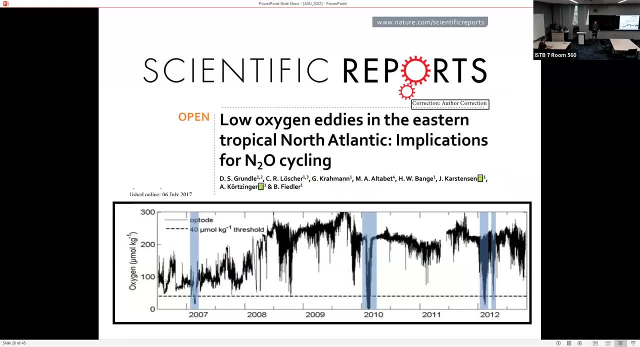 mangrove regions. So this gives you an example, idea of sort of the places we've worked, type of measurements we use. Before I sort of finish up, though, I wanted to at least take you through one story from start to finish, And I picked this one because one I think it's a. 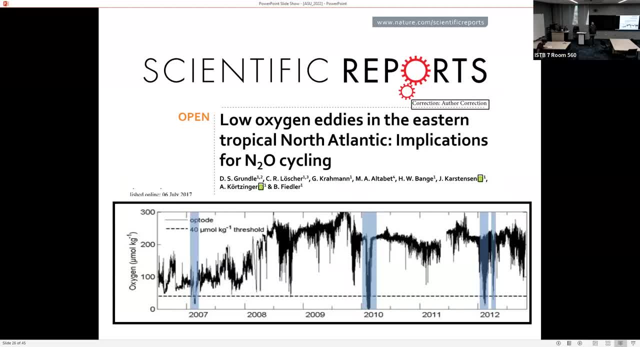 pretty cool. it was a kind of pretty cool new finding. But two, I think it's a pretty straightforward story to take you through in a few steps, especially for, you know, anyone That's not into the nitrogen cycling sort of you know process. So this is a paper that we 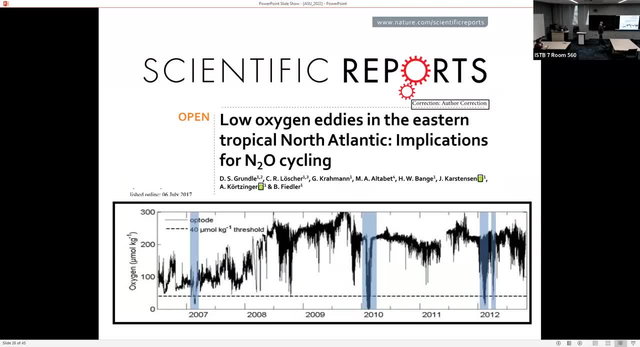 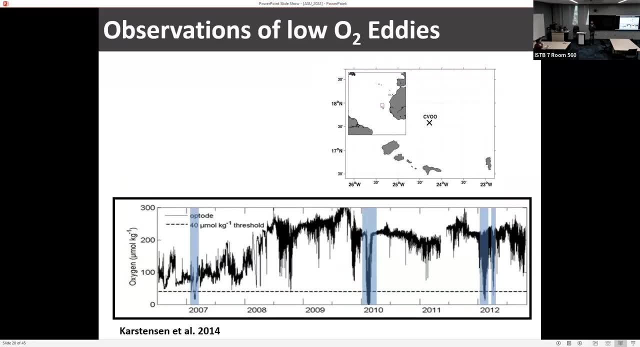 published titled Low-Oction Eddies in the Eastern Tropical North Atlantic and their Implications for N2O Site. Let me just give you a bit of background. So back from about 2006 to 2013,, colleagues of mine at Guillaumar had a mooring out of the Cape Verde Ocean Observatory, just northeast. of the Cape Verde Islands. here On that mooring at about 12 o'clock in the afternoon there was a very strong, fiery, Izzy employee. He was going to be very, very quick to take a look He was going to. take a closer look. So it's interesting. he was going to walk around the lake But before we could see him at the end of the day and see him, he was a little bit on the brink, but you can take a look at his. 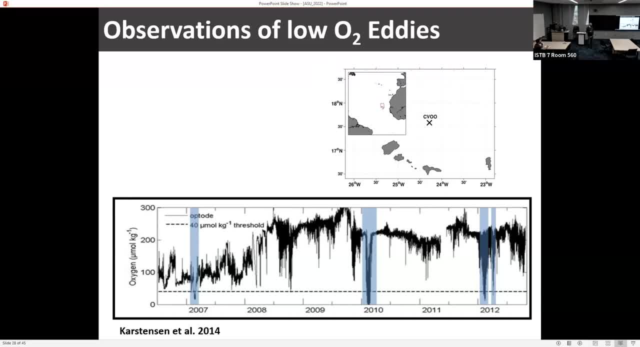 On that, mooring at about 50 meters depth. they had an oxygen sensor And when they compiled all that data, what they found was that- and remember I said, the Atlantic Ocean is always really well oxygenated. This is the exception. So when they compiled all this data, they found- highlighted in gray here- that every so often oxygen concentrations just drop down to, you know, close to or even to zero oxygen concentrations. 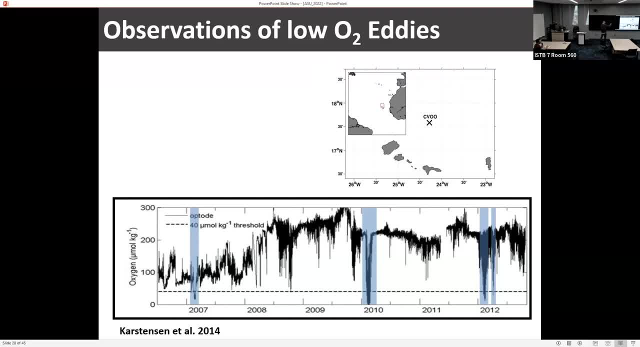 What they found was that every time one of these events occurred, it corresponded with an eddy passing through the region. So eddies are these circulating water masses that propagate through the ocean, and they can have very distinct chemical and biological signatures. 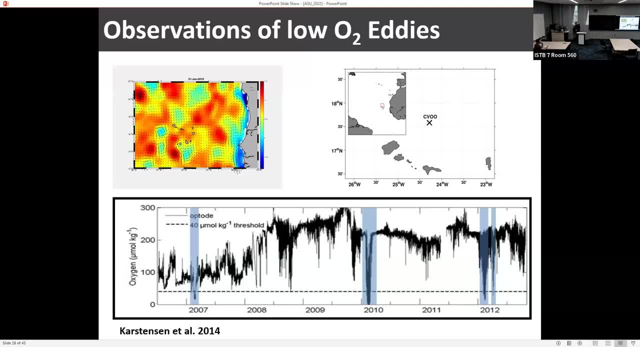 And this. let's just see if this is Here, you can just see these eddies. They're essentially forming off the Mauritanian upwelling system. They hook off here and start spinning and they propagate past the Cape Verde Islands. 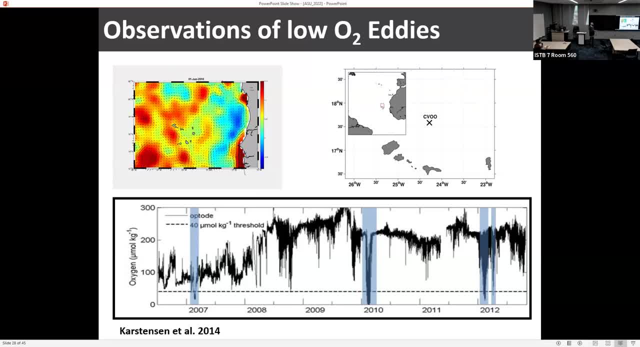 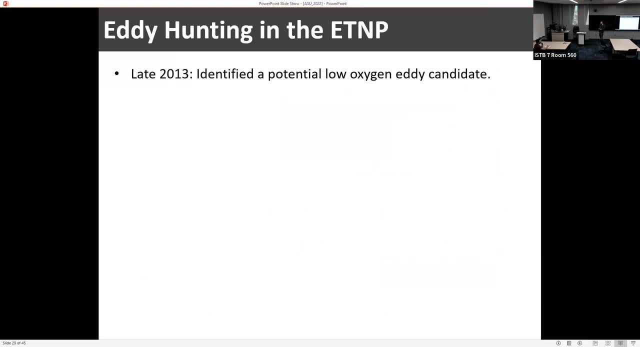 So the conclusion, or the thought, was that some of these eddies must be characterized by really low oxygen conditions. So when I got to Guillermar in 2013,, a few of us wrote a proposal to the Future Ocean Cluster of Excellence and we got awarded to go out and conduct a short eddy hunting survey and collect some. you know, make some measurements for different things. 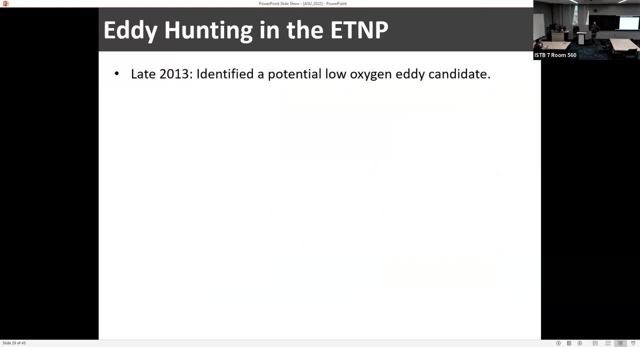 So in late 2013,, we started using satellite imagery to identify a potential eddy candidate- low-oxygen eddy candidate. Then, in early 2014,, we went down to Cape Verde. we deployed a couple of gliders. we were able to drive these gliders into this eddy candidate. 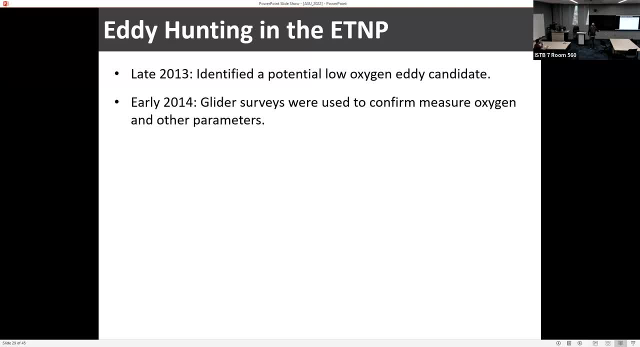 One of the sensors that was on that glider was an oxygen sensor, So we were able to- instead of having to go out on the ship and back and forth trying to find the eddy, we were able to use these gliders to go out and do the job for us. 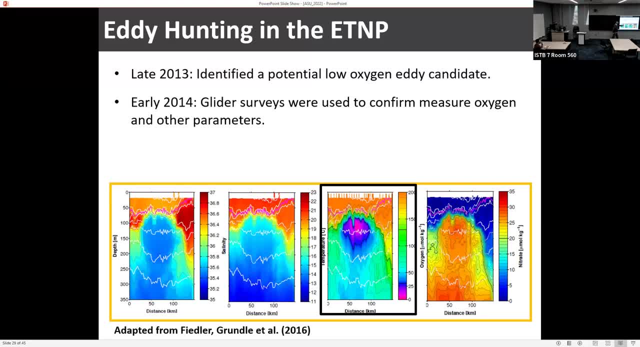 And you can see here. so we've got temperature, salinity, oxygen and nitrate. What I really just want you to focus on here is the oxygen, the third figure from the left, And when we look in the center of this figure we can see that we're getting this pool of really low-oxygen water in the core of the eddy. 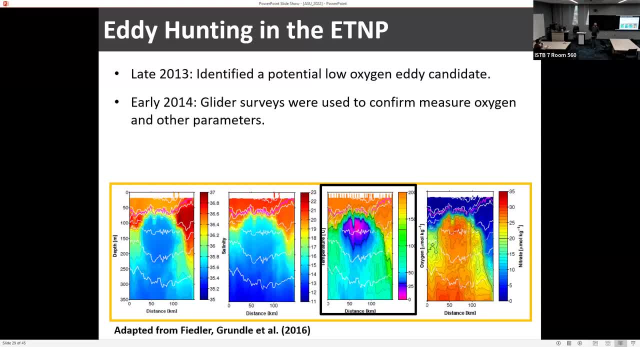 So this confirmed to us that yep, we've got a low-oxygen eddy. So now, in March 2014,, Bjorn Fidler and myself went down to Cape Verde to go out and do some research, And we were able to find this shipboard sampling this eddy. 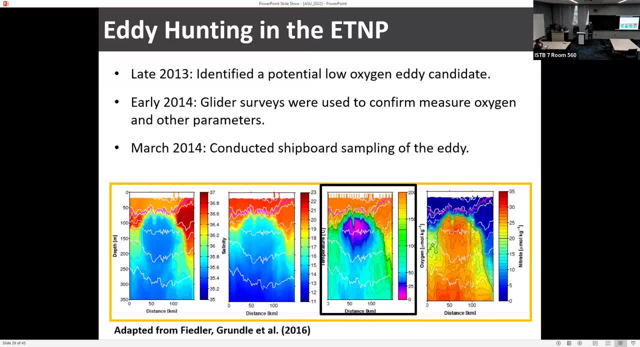 This was anything but trivial. We were using a very old, very broken-down Icelandic fishing vessel that had been donated to the Institute there When we first got there. I'm looking at the ship. the fenders are falling off, the ship's rubbing up and down as the concrete dock bits of it are falling off. 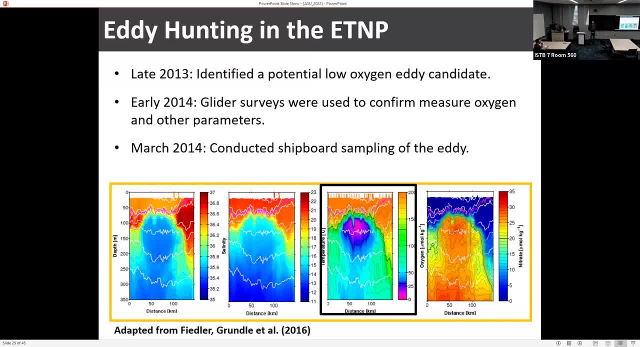 It took us a number of attempts. We were down there for like four weeks just to try and get out for a day or two of sampling. We finally managed to do that. looking at things like vertical migration of zooplankton, How are these dead zones or these low oxygen zones? 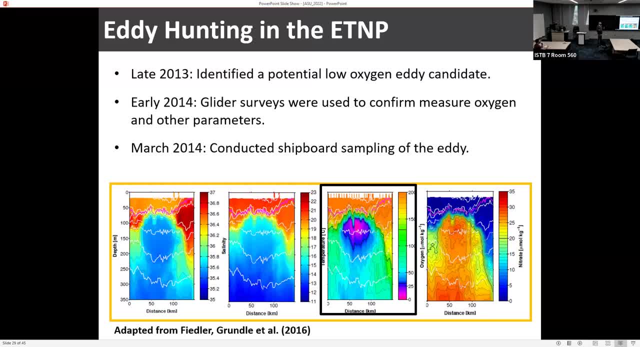 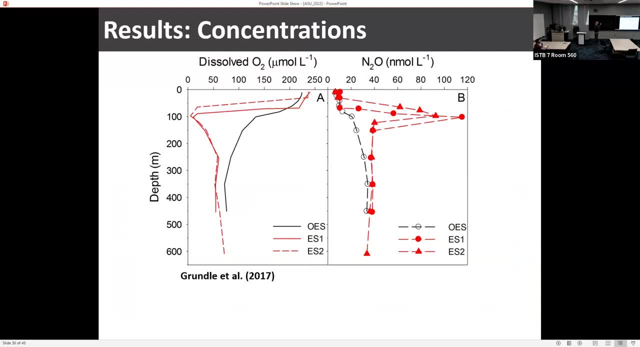 impacting that. We were looking at some of the physics, the carbon chemistry and then of course, nitrous oxide. So just to show you some of the results here. So we've got dissolved oxygen through the water column on the left, N2O through the water column on the right, 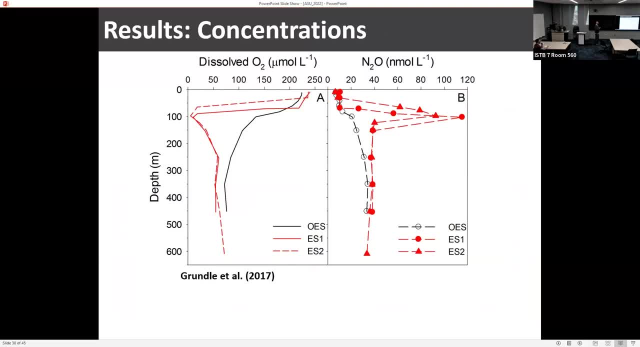 Black lines and black data points represent a reference station outside of the eddy, So our kind of typical conditions that we see in this region. red represents a couple of the stations inside of the eddy, So we can see again here the oxygen concentrations. 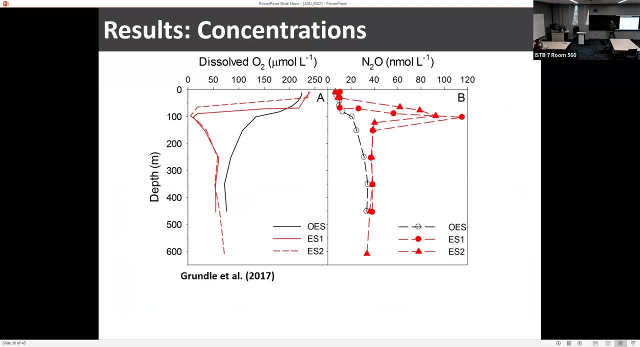 in the core of the eddy are really dropping off. One station, we were down to just under 10 micromoles of O2 per liter and another we were down to just under five micromoles of O2 per liter. Looking at N2O outside of the eddy: 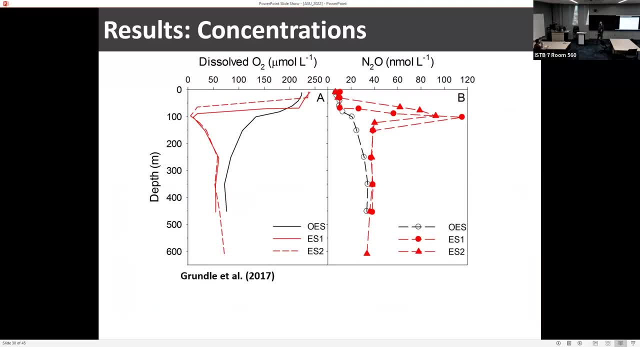 the concentrations are pretty much bang on what we see in this region And really anywhere in the Atlantic. they don't get much higher than about 40 micromoles, or sorry, 40 nanomoles, of N2O per liter. But inside of that eddy we were getting 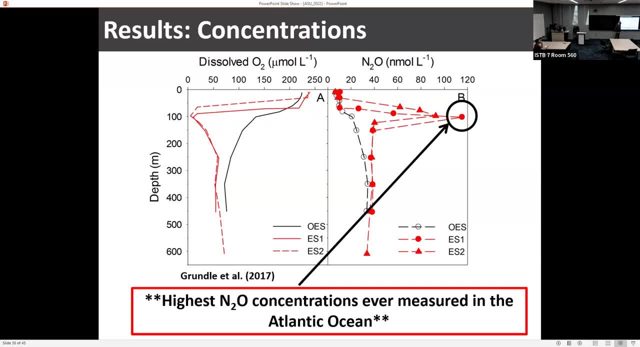 they just ramped up. in the oxygen minimum zone We were getting up to close to 120 nanomoles of N2O per liter, and this is by far the highest concentrations that have ever been measured in the Atlantic, and they're on par with sort of 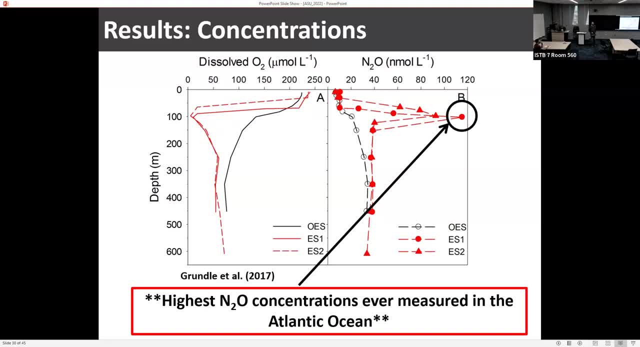 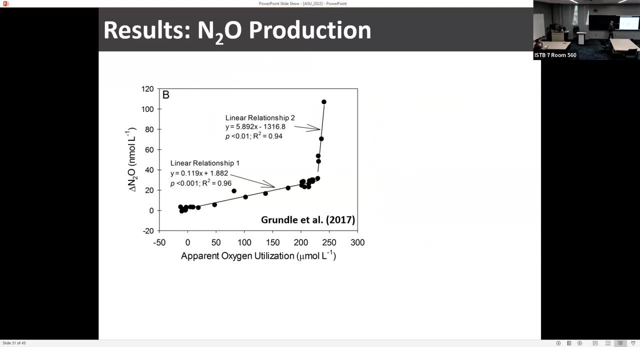 the high N2O concentrations that we see in the Pacific and the Indian Ocean. So again we calculated del N2O versus AOU And we found they had two very distinct linear relationships, which I just called relationship one and relationship two. 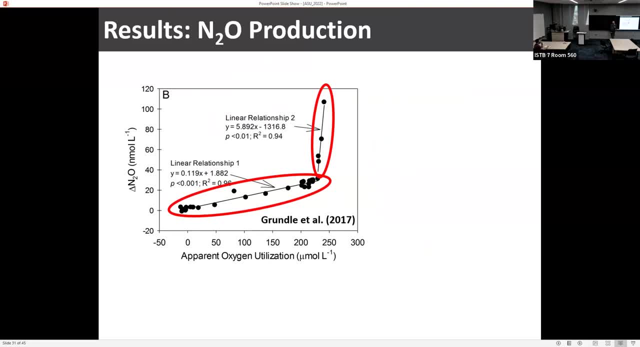 So this first one is an oxygen concentrations above 20 micromoles of O2 per liter. about 22 micromoles and above, We can see we're getting not a lot of N2O being produced versus oxygen consumed. But as soon as we drop below 20 micromoles of O2 per liter, 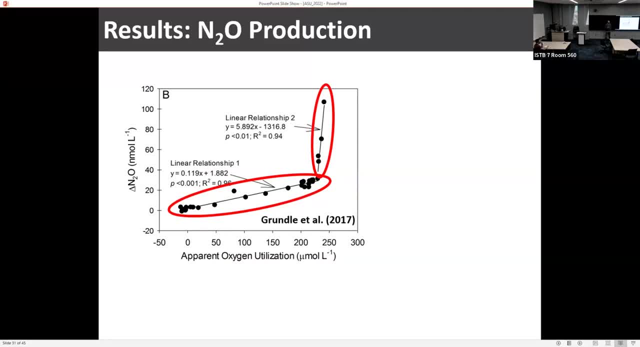 moles of O2 per liter, that N2O production really starts to ramp up. And if we look at the slopes of the relationships, we were able to say that above about 20 micromoles of O2 per liter, 8,500 moles of oxygen would need to be consumed to produce one mole of N2O. 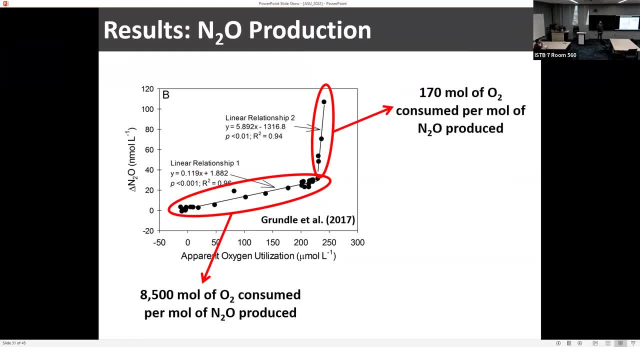 Below 20 micromoles of O2 per liter, we were able to say that now we only need 170 moles of oxygen to be consumed to produce one mole of N2O. Put in sort of maybe simpler terms, that's essentially: 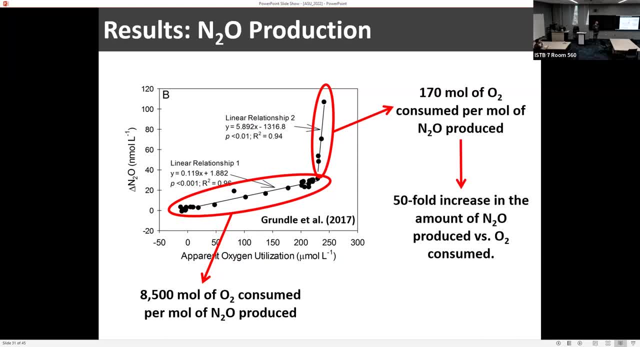 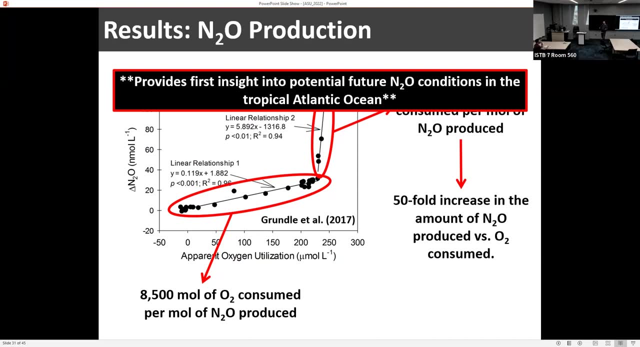 a 50-fold increase in the amount of N2O being produced versus the amount of oxygen being consumed As soon as we hit this threshold. it's a very sort of abrupt tipping point that we're seeing, And so, in addition to providing some information, some new information for the Atlantic. 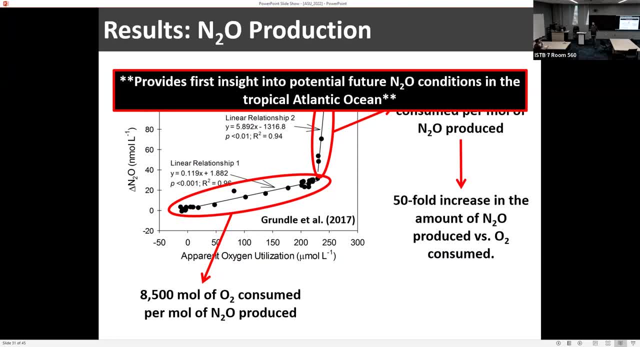 Ocean to say, hey, it's not quite as boring in terms of N2O as we thought it was. and we need to say, hey, it's not quite as boring in terms of N2O as we thought it was. and we need to say: 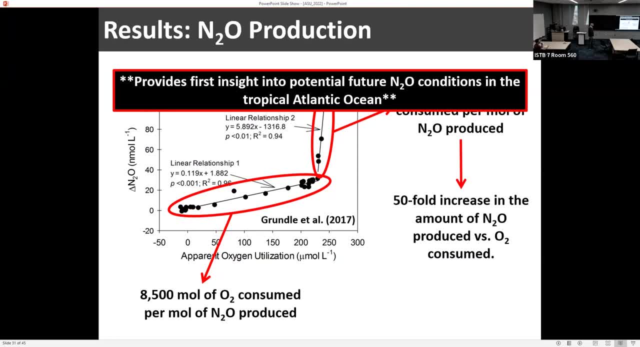 we need to say, hey, it's not quite as boring in terms of N2O as we thought it was and we need to start thinking, taking these eddies into consideration. But it's also again, we're using it as a natural laboratory to provide that sort of first insight into the potential N2O. 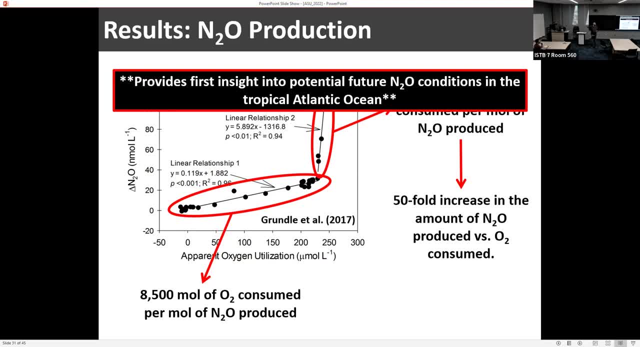 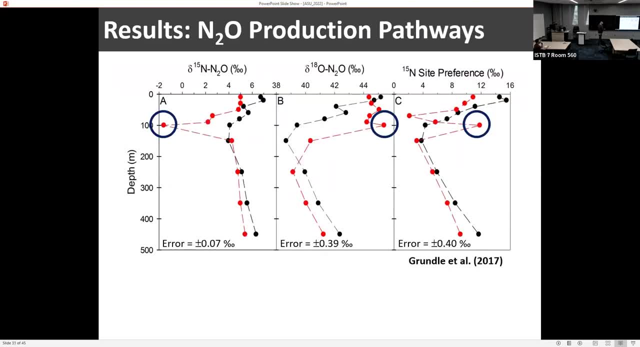 conditions that we might see in the tropical Atlantic Ocean decades from now, as we move through this century, if oxygen concentrations continue decreasing. I'm going to very briefly touch on some isotope results here. So we've got del-15N, del-18O and the 15N site preference. 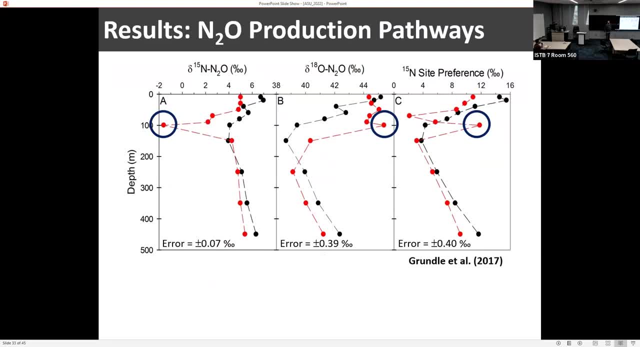 of N2O- Red is inside the eddy, Black is outside of the eddy, And what I really just want to focus on here is the circled points where we saw really massive changes in the isotope signatures, And this indicated to us that 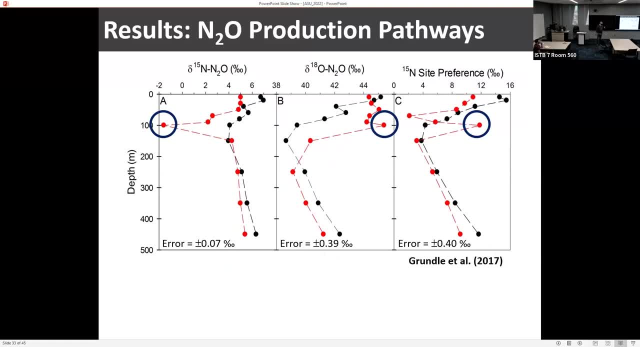 denitrification had started to become an important source of N2O, And I'm just highlighting this because I think this is another. this is kind of pretty cool as well. This is the first time that we've ever seen any evidence for denitrification water column denitrification in the Atlantic. 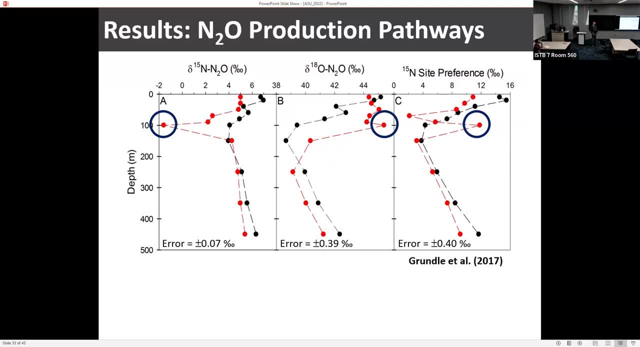 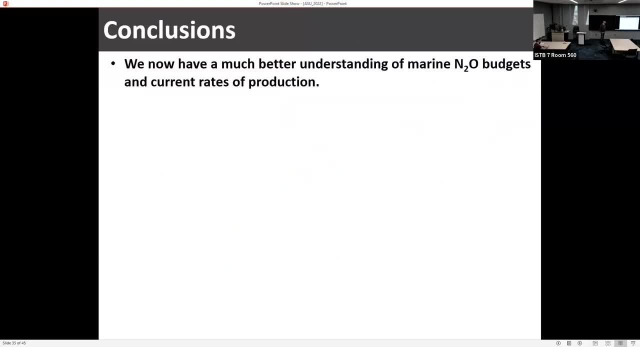 Ocean. So again, these eddies are pretty cool features to get out there and study. It's not easy, but it's certainly worthwhile. Okay, So just to wrap up with a few thoughts and concluding points, So not just from the low-option eddy, but from the work that we've done. 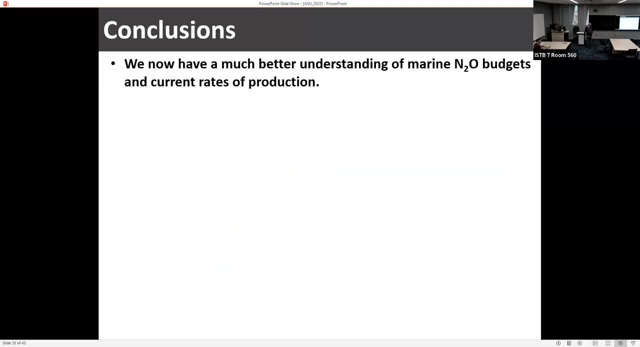 in other regions- in coastal regions, Atlantic regions, in the Pacific- and that colleagues might have also worked on. I think we now have a much better understanding of marine N2O budgets and the current rates of production in different marine regions, And these low-option regions that we've been studying really are ideal. 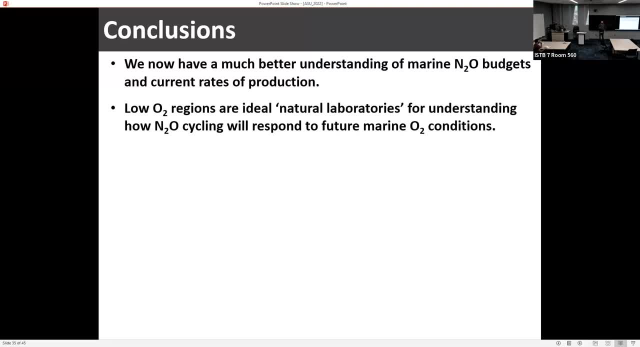 natural laboratories for understanding how N2O production could respond to future marine oxygen conditions. So I'm going to generalize a little bit here. It does vary slightly from region to region, but I think we can now begin to better constrain the oxygen thresholds. 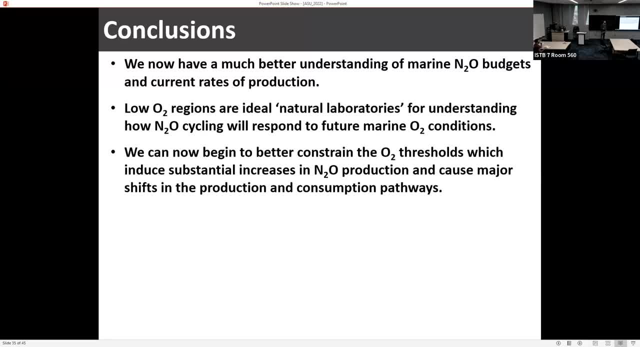 which induce substantial increases in N2O production and cause major shifts in the production and consumption pathways. So I think in general terms we can say that below about 20 micromoles of O2 per liter, N2O production really starts to increase And you've seen just by how much it can increase Below about. 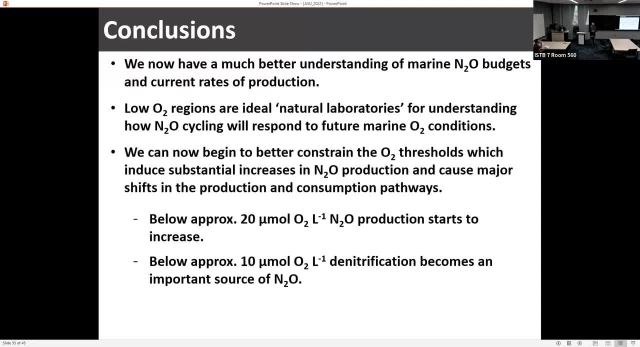 but it's still. nitrifying bugs are the ones that are really producing it, whether it's through ammonium oxidation or nitrify or denitrification. Below about 10 micromoles of O2 per liter, denitrification becomes an important net source of N2O, And then somewhere, 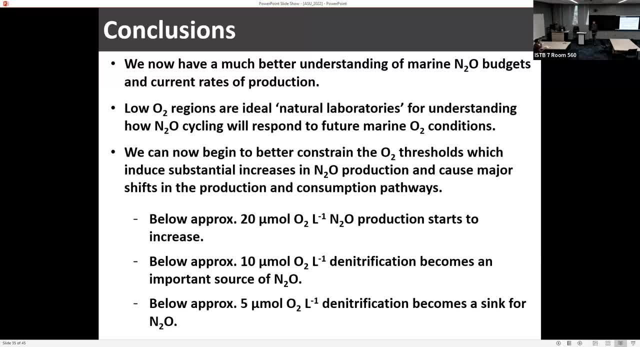 between that's a bit below five micromoles and zero micromoles of O2 per liter denitrification become a sink for N2O. So I think these results that myself and other colleagues have been coming up with really are useful. We now need to start using them to inform the biogeochemical. 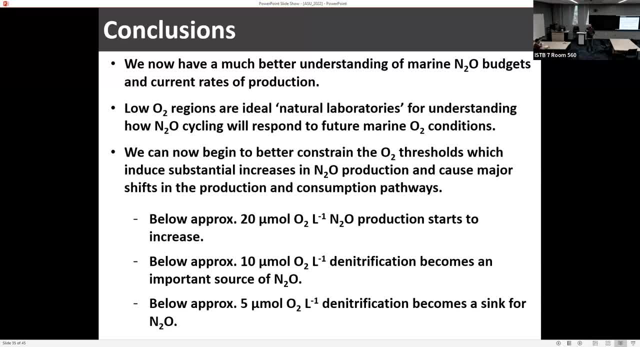 models, People that are sitting there trying to predict what's going to happen with oxygen in the future. we can now start plugging in some of these findings into those models to start predicting how much N2O will be produced, or when's the tipping point, And then we're. 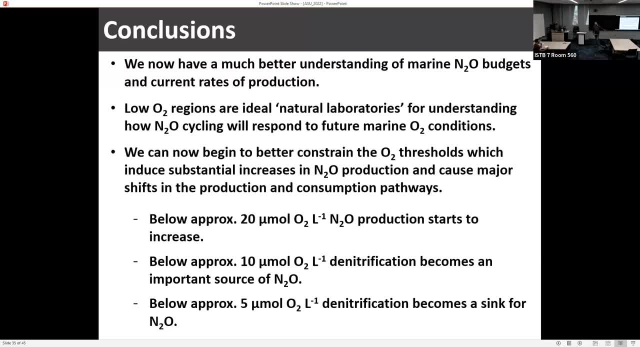 going to start looking at what's the tipping point going to occur. It's not quite as simple as that. There's a lot of complexity there. We've got to think about feedback mechanisms. You can imagine if we've got more N2O going to the atmosphere and the atmosphere is warming. 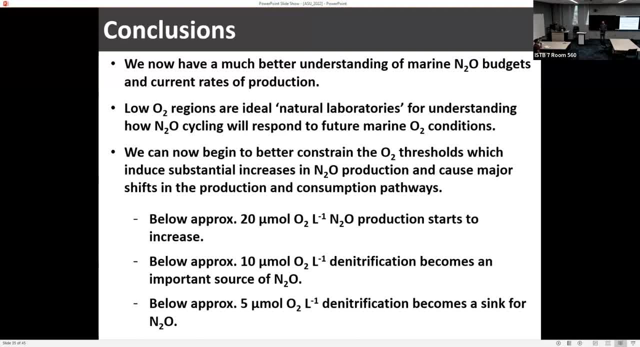 more, then we're going to have more stratification, We're going to have less oxygen penetrating down to depth, We're going to. oxygen is going to. consumption is going to speed up, And we can think about these in multiple different ways, but there are a lot of. there's a lot. 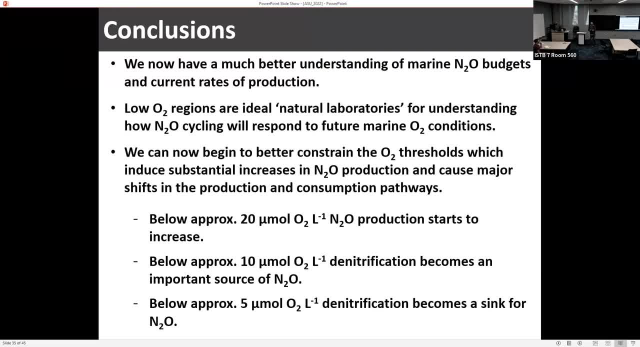 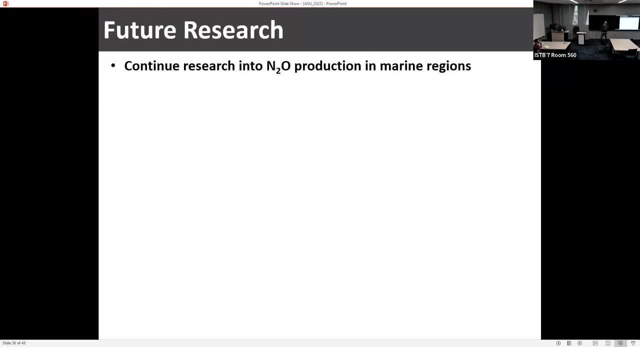 of complexity here. It's not just as straightforward as plugging this into a model, but you see where I'm going, Okay, So just now, spend the rest of my time just thinking about some future research plans. So, just because I said we've found some really cool results so far and we've got a much 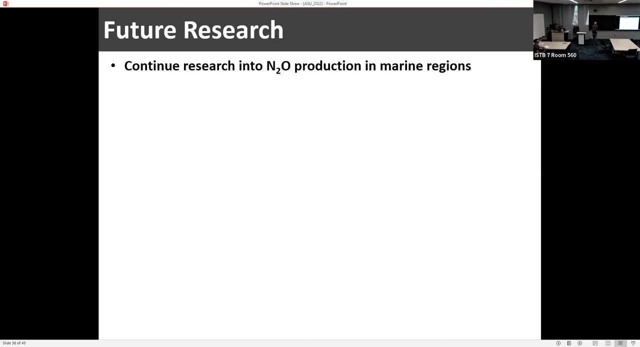 better understanding of N2O production doesn't mean we should stop looking at this. We need to continue this in other regions. We need to start looking at other environmental variables. you know quality, Quality of DOC, for example dissolved organic carbon. You know, I will say: could you imagine? 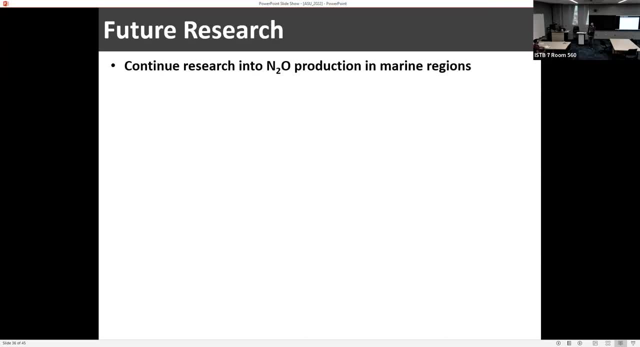 if we stopped measuring primary production in the seventies, we just wouldn't have the same understanding as we do today- the primary production in the ocean- and we wouldn't have been able to sort of track those changes as well. So we do need to continue with this. 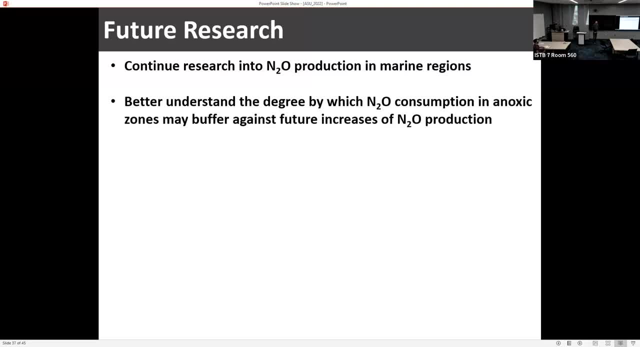 work and we will continue with it. The thing that one of the other things I'm really interested in here is that a lot of us have been working on this topic of energy. We've been working on this topic of energy for a long time now and I'd like to think about the effects of this on the energy economy. 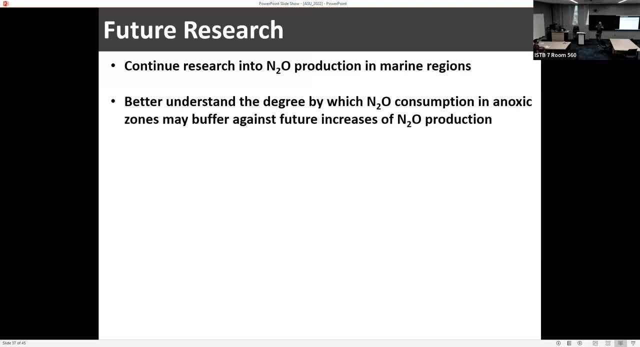 and energy production. So that's one of the things I'd like to think about as we go forward. I mean, there's been a lot of work in the end of the last decade, for example, with the environmental power and the energy production- the energy production in the ocean- But we 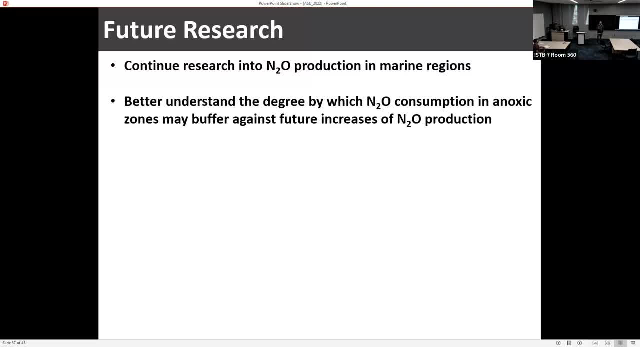 do have N2O consumption and anoxic zones occur. So you can imagine, if these hypoxic or low oxygen zones in the ocean expand, we get more N2O being produced. But what if the anoxic zones where we've got denitrification consuming N2O also expand? in science It may act to buffer, at least to some degree, against those increases in N2O production. The trouble is we really don't have much of an understanding about this. 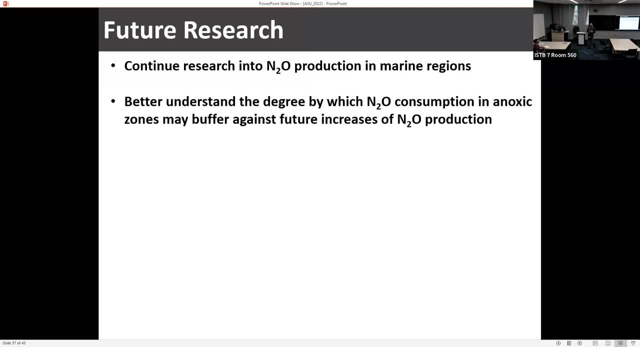 So I wrote a proposal with NSF that was funded recently with my co-PI, Frank Stewart, and we're going out trying to investigate this. We just finished- recently finished- our first sampling campaign in San Aginile. Getting back to San Aginile, it's just an awesome place. It's easy, easily accessible. 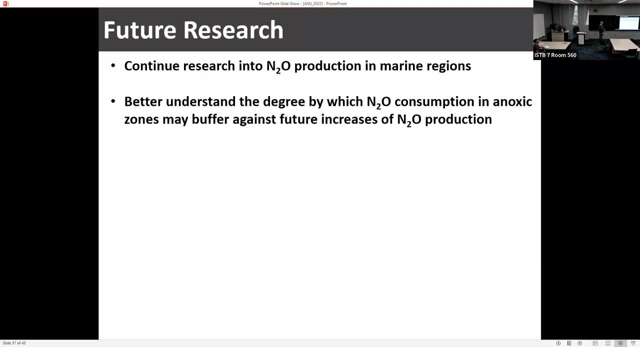 It's got predictably low oxygen concentrations. So we've been out, we've started this and just want to show you some very preliminary results. I just got these a few days ago. This is from one sampling, just one of our sampling days in San Aginile, at just two different stations within the inlet. 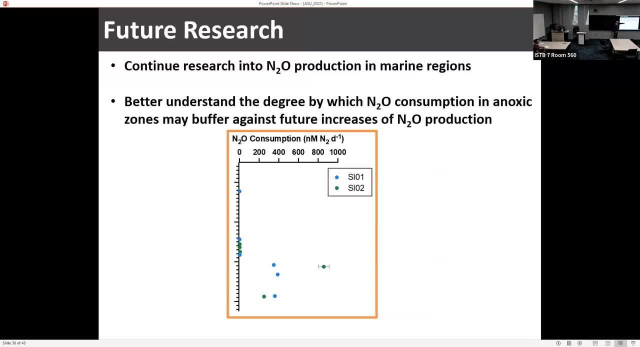 And I'm realizing that the depth hasn't shown up here. but basically we're going from the surface down to about 200 meters depth. So when we've got oxygenated water, even at the hypoxic, anoxic boundary, we've got no N2O consumption occurring. 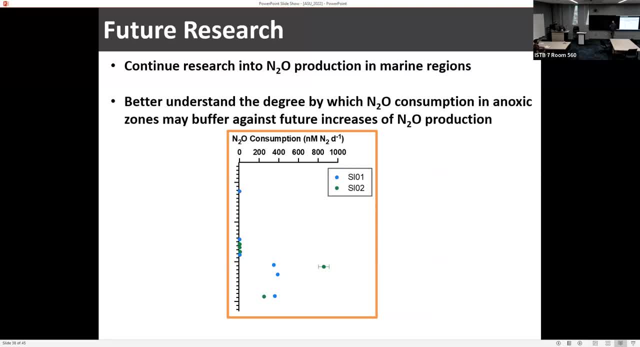 But as soon as we get into the anoxic zone we see N2O consumption really ramping up And basically, just doing a quick calculation in the last couple of days, I think the kind of rates of N2O consumption that we're seeing. 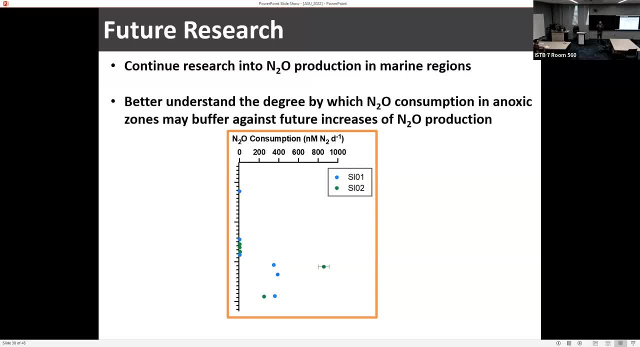 they could certainly consume any N2O that's diffusing from the overlying waters down to the anoxic zone about as fast as it's coming at them. So this is certainly good. It's certainly giving us some idea that denitrification in anoxic zones can act as a buffer. 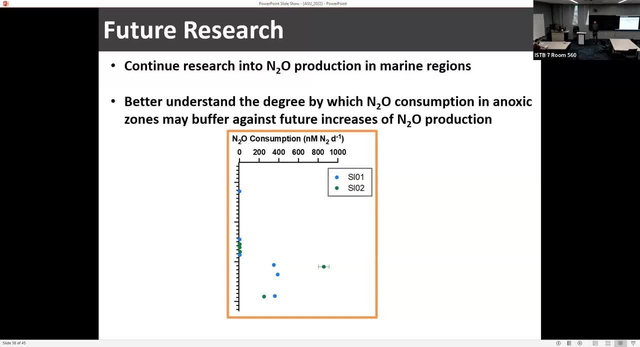 We don't know what degree yet. That's going to be worked on over the next sort of two, two and a half years still. Another topic which I'm interested in is this idea that sulfide can inhibit N2O consumption, And I'm working on a proposal that will be submitted to NSF in about two weeks time to look at this. 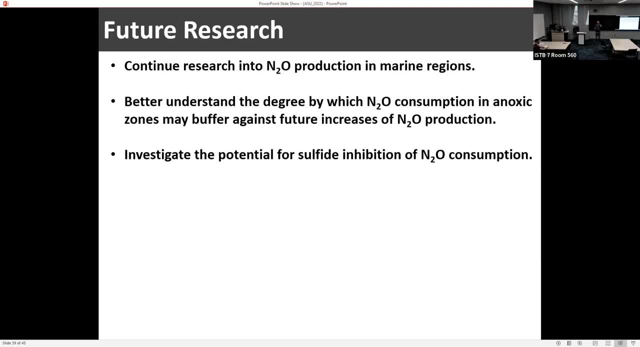 So the idea is that, OK, we've got this where it just adds layer to layer, of complexity right Becomes a bit more complicated. So we've got these low oxygen zones where we've got N2O production occurring. We've got anoxic zones where denitrification can consume some of that N2O that's been produced. 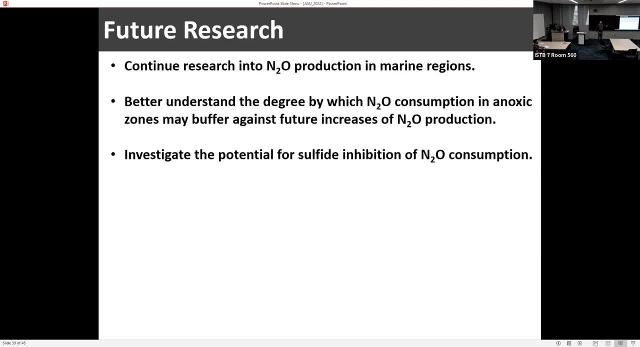 But in anoxic regions at times we see sulfidic events occurring. So if that's preventing denitrification from consuming N2O, we need to understand this as well. And just to give you an idea, this isn't the only evidence, but just a quick figure that I put together over the weekend. 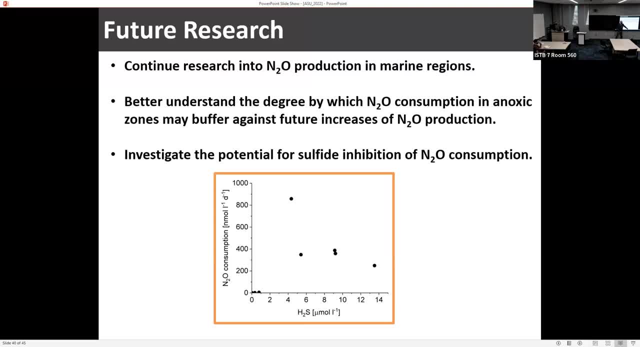 This is N2O consumption on the y axis. hydrogen sulfide concentrations on the x axis. We've got these very low sulfide concentrations. This is basically the hypoxic, anoxic boundary where we don't have N2O consumption occurring anyway. 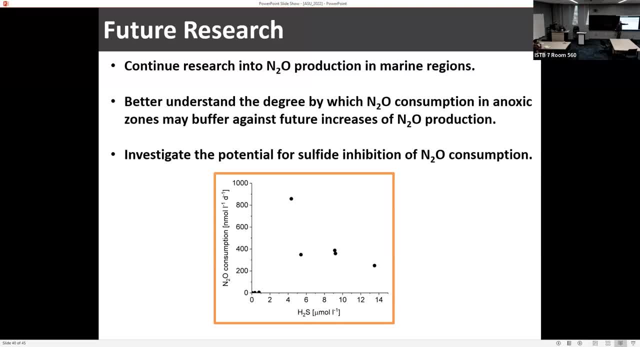 We get into the anoxic zone, N2O consumption really increases. But then when we get above about five micromoles of H2S per liter, we see that N2O consumption slowing down. It's not completely inhibited, but it does seem to be slowing down. 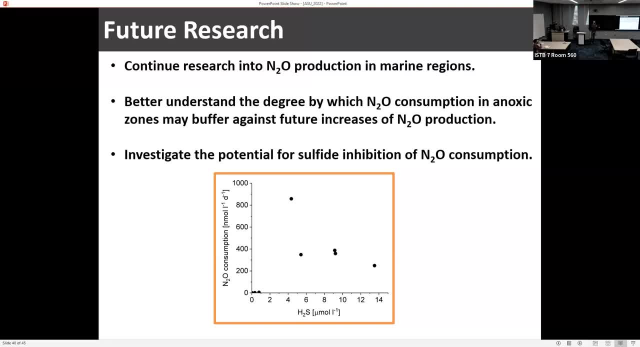 And just so you know, it's not because it was less N2O. The N2O concentrations were actually experimentally manipulated and kept them all sort of the same. So that's another topic that I think is worthwhile, And again, I'm working with Frank Stewart on this. Frank is my collaborator. 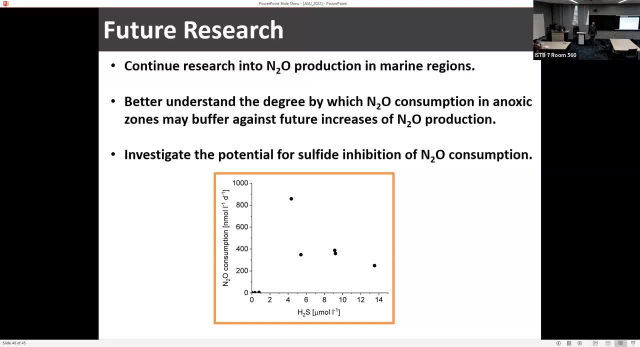 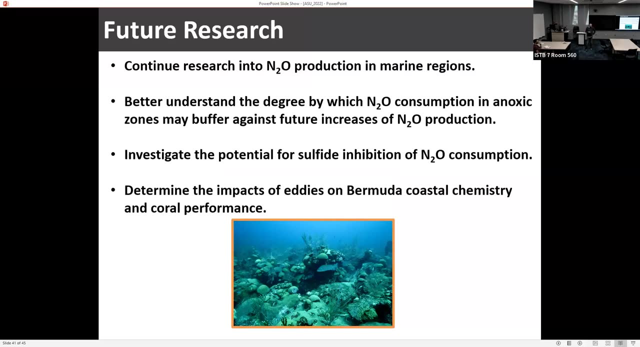 I work with a lot for the molecular genetic side of things So we're hoping if that was to be funded that would start up early next year. Yvonne Saval, myself and our co-PI, Natalie Goodkin, were just awarded another NSF grant to start looking at the impacts of eddies on Bermuda coastal chemistry and coral performance. 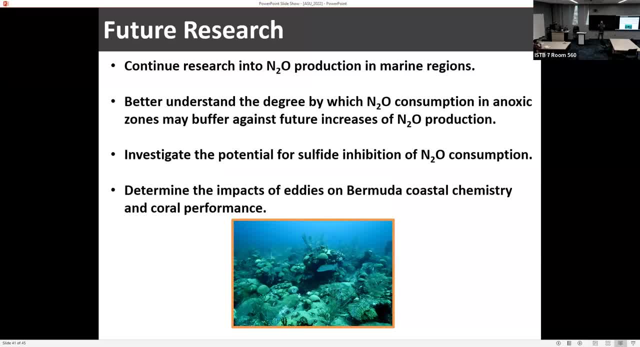 So again we've got these circulating water masses that have fairly distinct, or you know, different, chemical signatures. What are those chemical signatures? Is those eddies sort of hit Bermuda, basically? And then what's the from Yvonne's side? what's the impact on the corals? 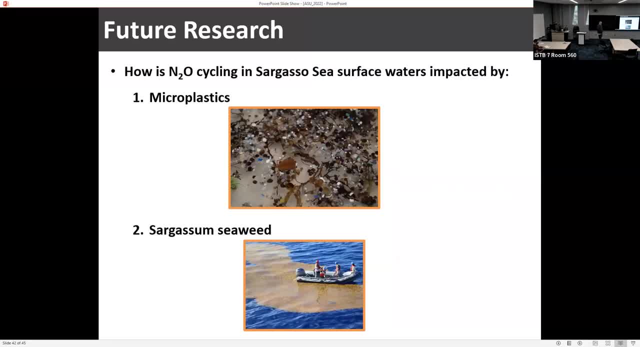 I think she'll talk about that a bit more tomorrow. And then a couple other ideas I've got. you know there's a number of other ideas that aren't just nitrous oxide, but I figured because the talk was nitrous oxide. I'll stick with this. 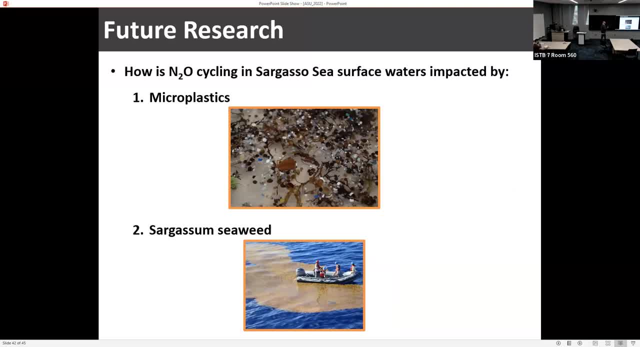 But looking at how N2O cycling in the Sargasso Sea surface waters could be impacted by N2O Things like microplastics, where we see a lot of microplastics in the Sargasso Sea off Bermuda, And then we also have these large Sargassum seaweed patches. 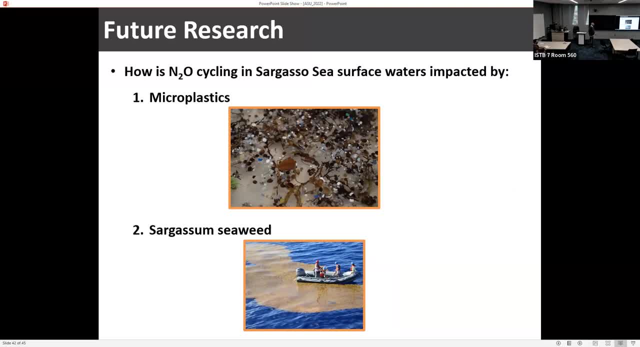 Hence the name: the Sargasso Sea. So you know, these kind of things like microplastics and Sargassum are they creating, are they able to sort of create these conditions where you can sort of get these buildup of biofilms of sort of you know? 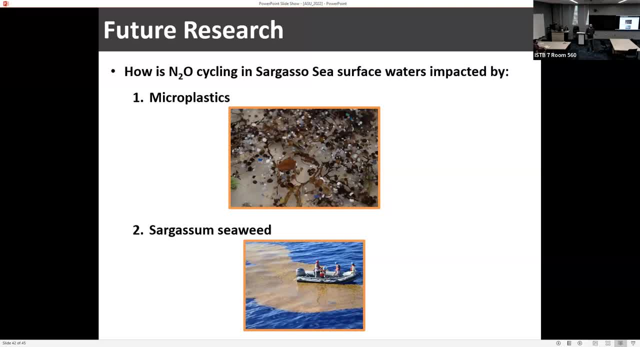 of the sort of bacteria in the archaea that are producing N2O, And do we see suboxic microzones forming where we might see more N2O being produced? We I've gone out and I've taken N2O concentration measurements in the Sargasso Sea. 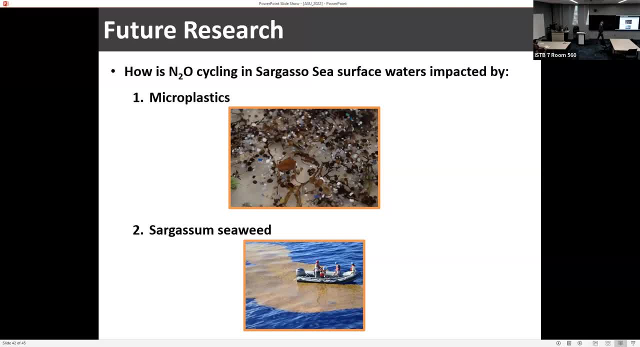 They're very low. But the point is, if it's right at the surface, where these things are promoting N2O production, we're not going to see it through a concentration measurement because it's just going to be ventilated straight to the atmosphere. 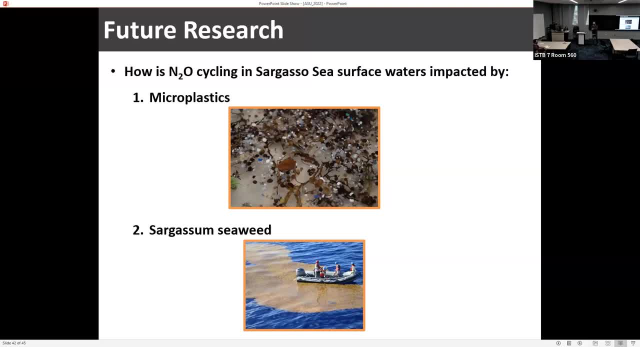 So I've been talking to Rachel Parsons, who's a senior research technician at BIOS, who's had a lot of- you know, done a lot- of work with microplastics and seaweed and is really interested in this, looking at the molecular side of things. 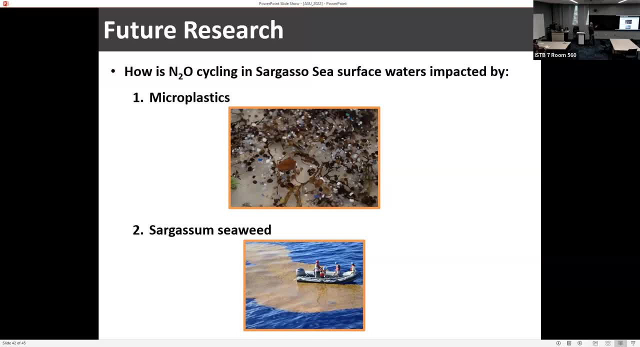 I've also been talking to Suzanne Neuer about microplastics. Suzanne has a lot of experience working with microplastics and we're planning to meet in a couple of days to discuss a potential proposal that we'd like to put together. And you know, I think the thing that we need to do is really sit down and think about the experimental approach here. 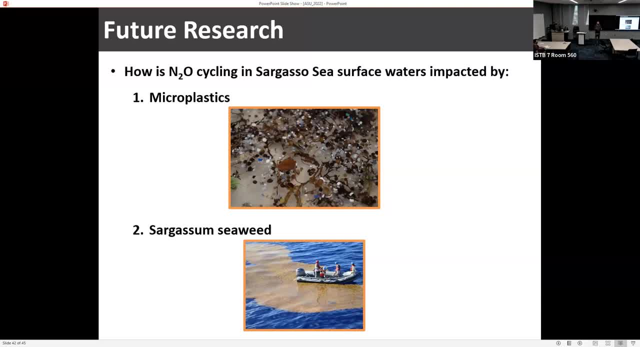 How are we going to, how are we going to identify whether there's N2O being really produced without one disturbing these systems too much? You know, I think it's going to be a combination of lab and field studies in this, where we're going to need to go out and collect, incubate and get back to using the 15N tracer techniques to look at this. 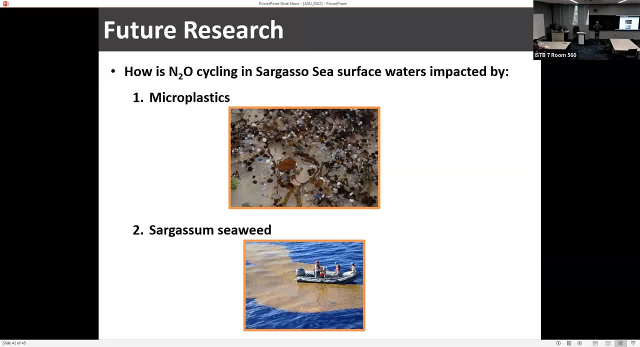 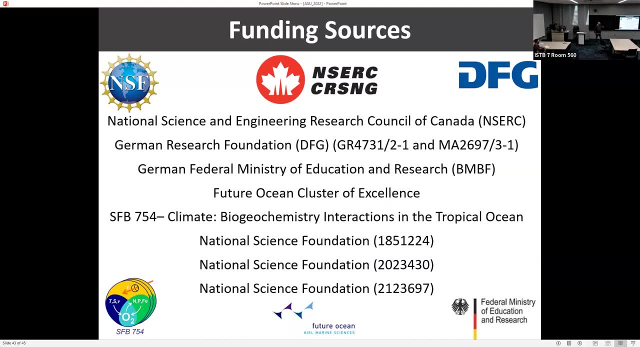 So With that I can wrap up. and well, I'll just, while it's up there, better acknowledge my funding sources, So everything from sort of NSERC in Canada to, you know, German Research Foundation and the Ministry of Education and Research which funded our Astro-OMZ crews. 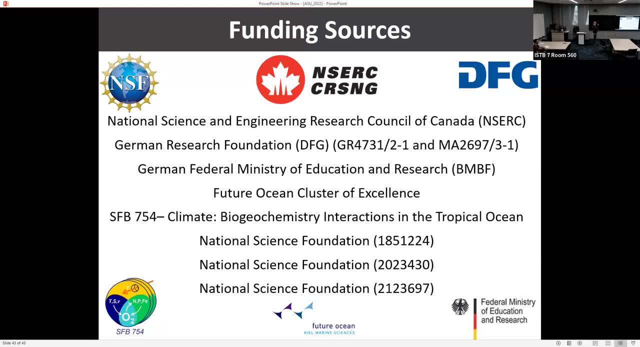 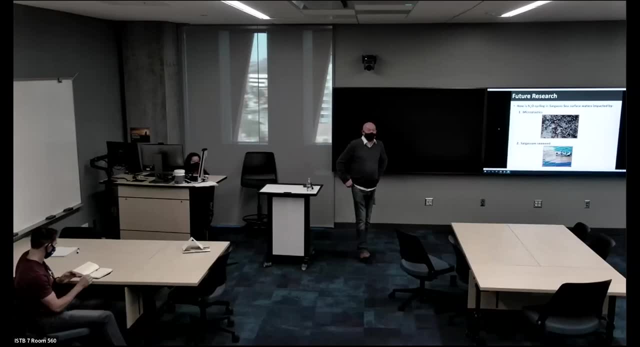 The Futurosa Cluster of Excellence in Kiel, SFB 754, and then obviously the National Science Foundation as well, And I'm happy to take any questions. If anyone who's online wants to type some questions in the Q&A and then you just go ahead and build questions here in the room and I'll look out for the Q&A and read those, the online questions. 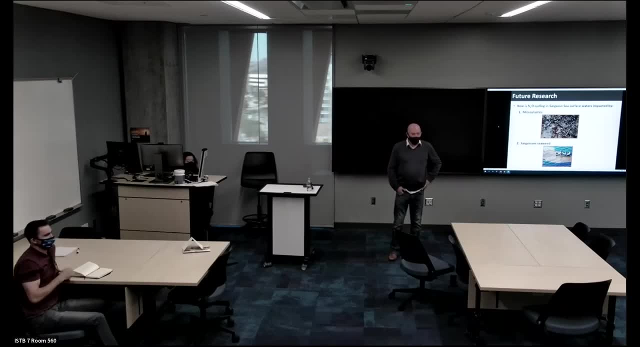 Great. So thank you for a great talk. Oh thanks, We don't get deep dives into biogeochemistry, right? No, I really appreciate that. I have a simplistic and it's actually probably a naive question, but a lot of the N2O production data you showed us was plotted against AOU. 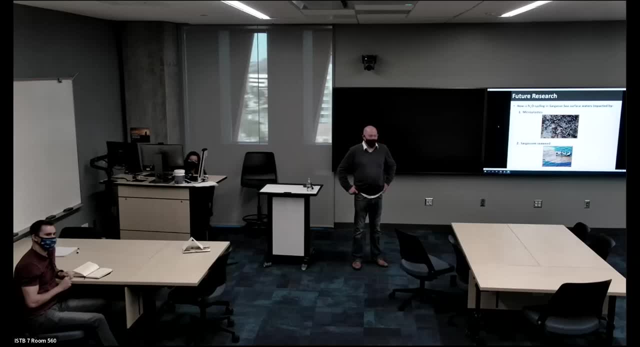 And the tipping point you made clear over and over again is when oxygen concentrations are extremely low or not, but that's when AOU takes off. How do you have apparent oxygen utilization when there's no oxygen? Yeah, So it's. 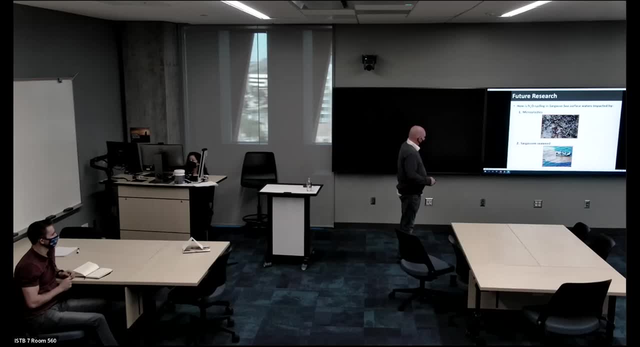 Let me just see if I can talk about that. So we're not really getting any more AOU, but certainly if we get a bit of sulfide you can start to get negative oxygen concentrations essentially, which will show up in a higher AOU. 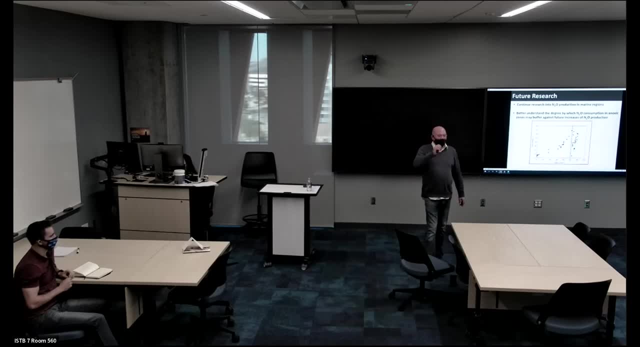 Negative oxygen concentrations. If sulfide is present, you start to kind of get into a position where You need more oxygen just to get back to zero, because the sulfide will just sort of poison that oxygen. It's not something I'm. 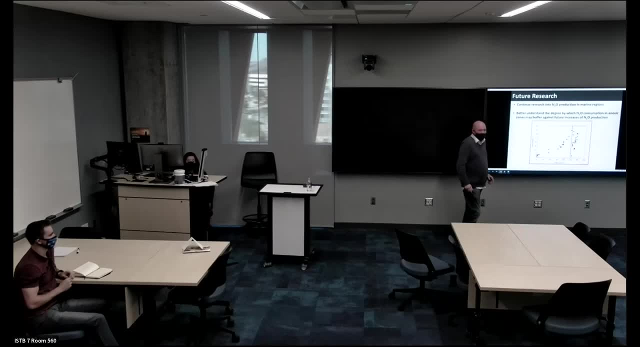 I've just, You know, somebody was just explaining that to me a while back, but But yeah, I mean some of this is also just due to probably some errands, a bit of diffusion. So some of this, This might not strictly all be the anoxic zone. 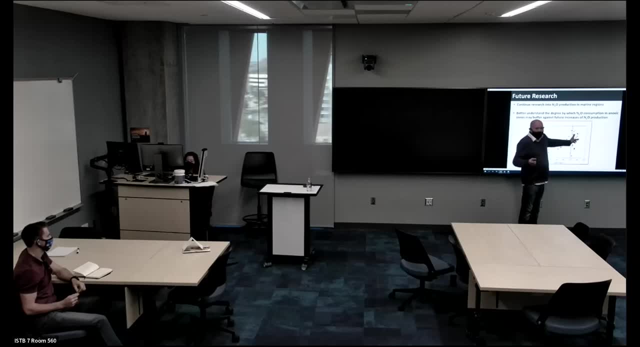 Some of this could be nitrifying And I think we've seen some of these N2O consumption signatures that have actually diffused into the boundary, the hypoxic-anoxic boundary. So maybe the anoxic zone is really sort of right here, where we don't see any more oxygen consumption occurring, but we're really seeing the drop-off of N2O. 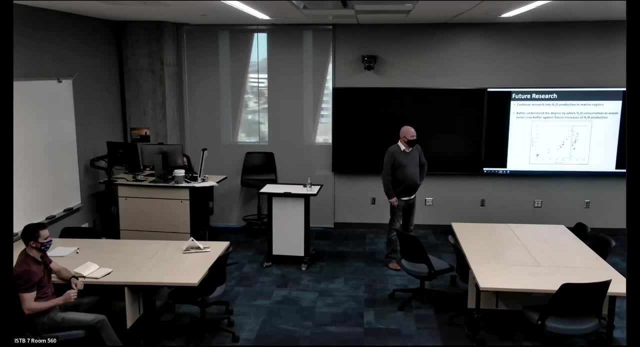 Yeah, Sorry, I'm not sure who was first there. How much of marine N2O? How much of marine N2O production comes from anthropogenic nitrogen deposition from the atmosphere and discharge in rivers. Is that causing an increase? Not really any. 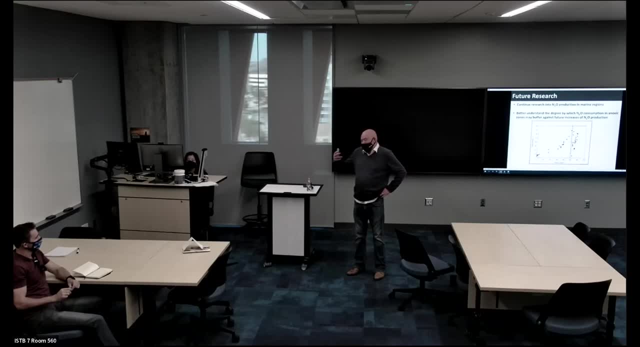 We do have anthropogenic N2O released from soils, from industry. I mean some of it you could say is anthropogenically derived. if you're pumping ammonium into a system And that's creating an anoxic condition and then 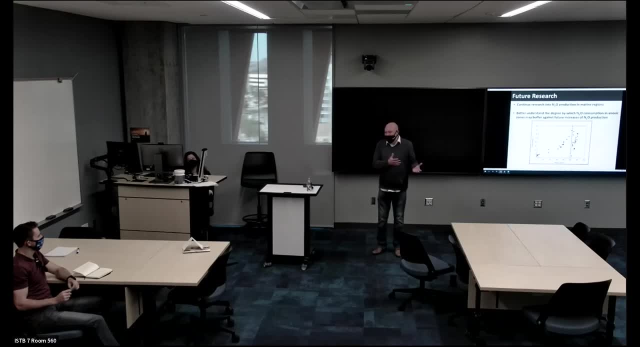 Or a suboxic condition, And then you're getting N2O production. You could say that's anthropogenically derived. I guess, from the standpoint of it's, The substrate has started off as an anthropogenic source or a pollutant if we get into coastal regions. 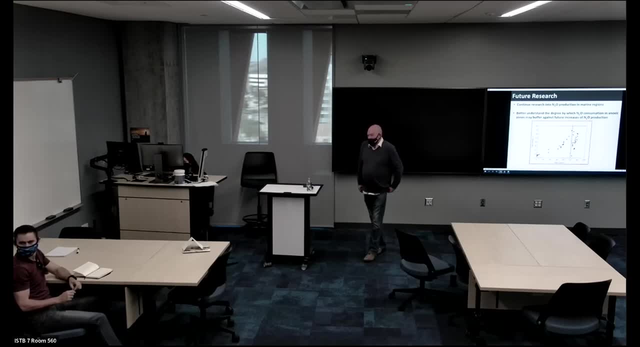 But, yeah, But the mechanism is mostly the impacts on oxygen concentrations rather than an increase in N sources. Yeah Well, that said, I mean no, Because if you're in a coastal system and you're really pumping, loading it up with ammonium, you're going to get N2O. You're going to get more phytoplankton growing. You're going to get more organic matter settling out. You're going to have more bacterial consumption of that organic matter, more oxygen consumption. So you're going to have- You are artificially driving down the oxygen concentration. 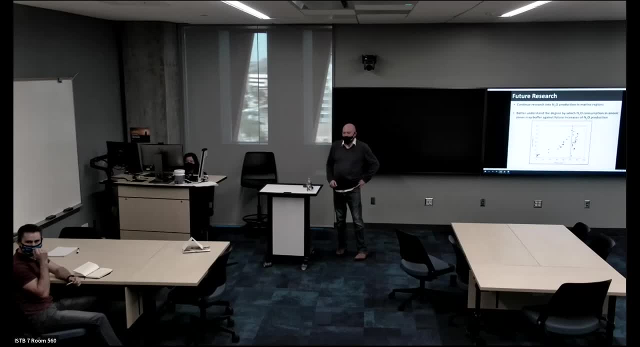 Right, We have another question. It's been said online that they can't hear the questions very well, So after you ask the question perhaps we can repeat for the online audience. For you working in Peru, have you guys looked at El Nino and La Nina events? impact on production. 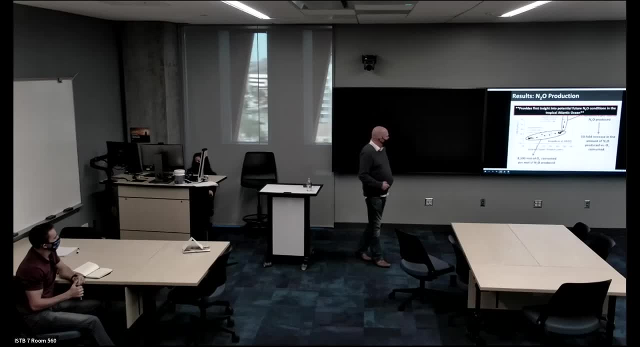 Yeah, Actually, we were So in this. I didn't want to get into it. I wasn't going to get into it just because it wasn't sort of the time, But this cruise that we ran in 2015 happened to be just as an El Nino event was really starting to ramp up. 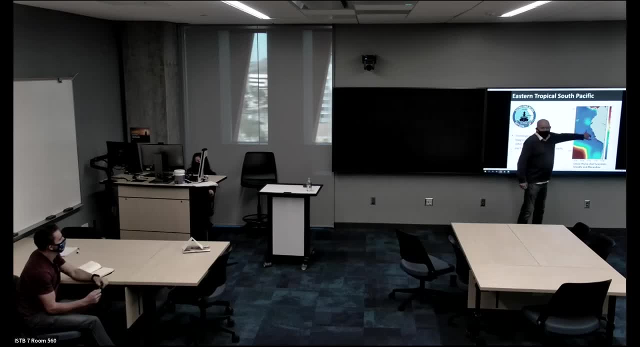 And we did. We published a couple of papers on this, So one looking at the sort of impacts that the El Nino had on nutrients, but also on the impact that it had on nitrous oxide, And let me just think about which way around this went. 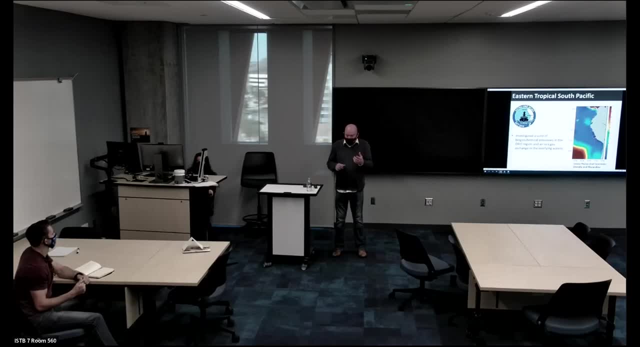 So what we were finding was that we were having There was less. The anoxic zone wasn't as well defined as it typically is, So we were getting more N2O. It wasn't necessarily the N2O production rates were higher, but the consumption was less. 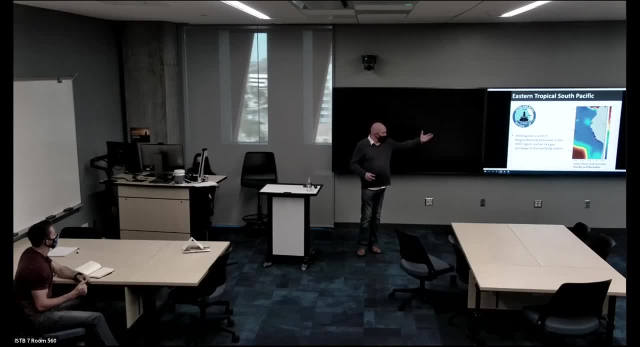 So when we had this El Nino event and compared it to previous cruises that we've had in this region, we were able to show that we actually had more N2O because we were not getting as much consumption. That zone of consumption wasn't as large as it was. 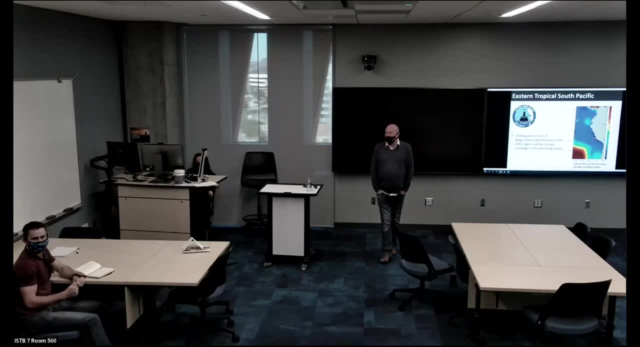 Sorry, Peter. Back to the question about oxygen utilization. Are you strictly working with utilization or are you also looking at the rates? Well, we do sometimes look at rates, But more, Not in great detail. It's more to kind of confirm that we're not getting, let's say, large changes in oxygen over the course of a several-hour incubation. 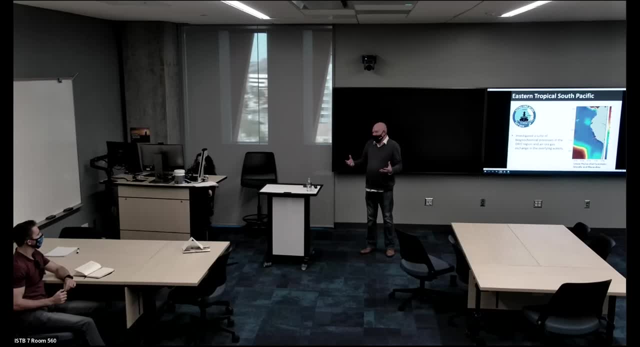 But no, we're just taking oxygen concentrations and calculating an AOU from that. We have something online. Hillary Hartnett would like to say thank you for a lovely presentation And she wonders: do you see N2O consumption all the way to the sediments in Saanich or only just below the oxic slash, anoxic interface? 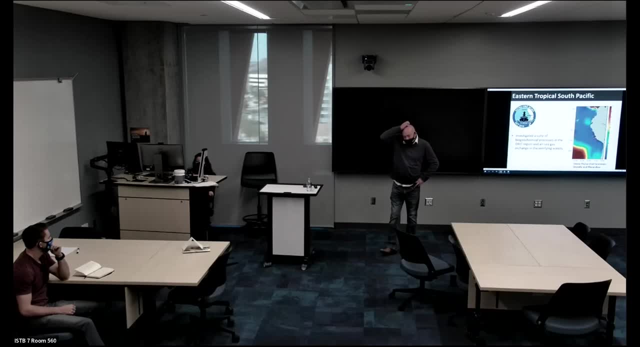 No, we see them all the way down. I'm still, And it's certainly going to be occurring in the sediments in Saanich and Lepp. I've been taking samples from close to the sediments. I'm not sure what to do with them yet. 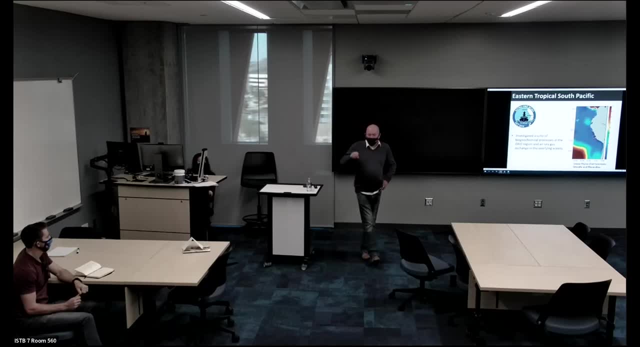 I want that data, but I'm not sure it's going to be very easy to incorporate into this story of using Saanich as sort of something that we can extrapolate our findings to other regions, Because if you've ever been down in Saanich and Lepp, the sediments start 10 meters before the actual like gets hard. 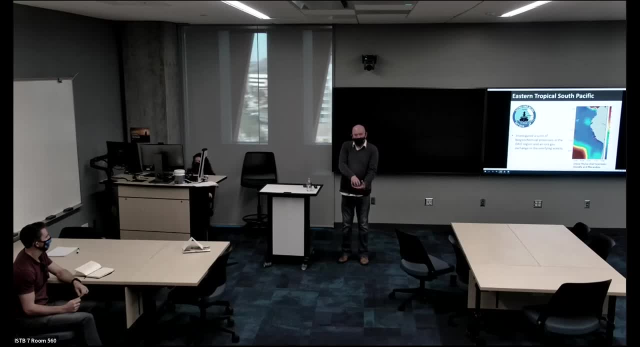 It's like just a soup, And you know. so I'm trying to avoid getting any contamination of samples for one And two. I don't want to, you know. I don't want to confound results from N2O signatures that are coming out of the sediments with what's actually happening in the water column. 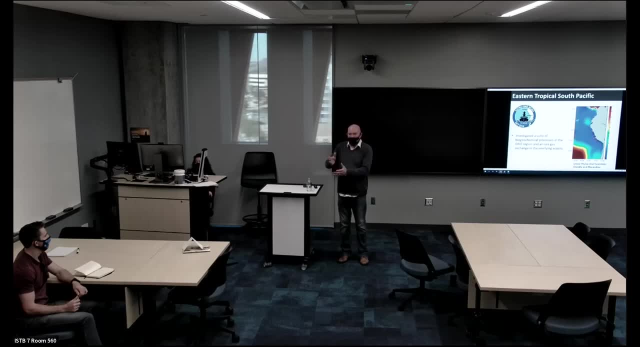 So we are taking that, but I'm not going to necessarily use it as much. in just identifying what's happening. in the water column We have another one that says great talk. Damien, What are your thoughts on future trends of N2O production in a world of declining oxygen concentrations in the ocean? 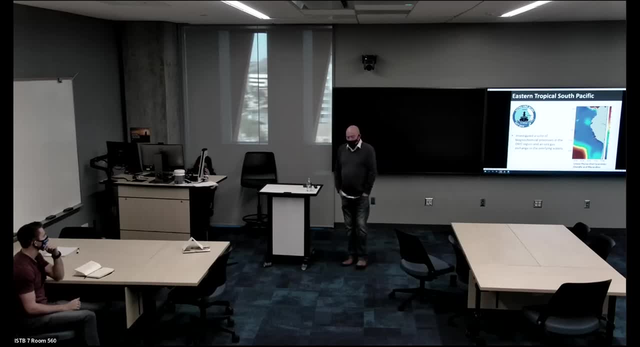 Yeah Well, I certainly think you know we're going to hit a point at some point through the century. This is something I really need to sort of maybe sit down with. I don't want to start giving you a year or a decade. 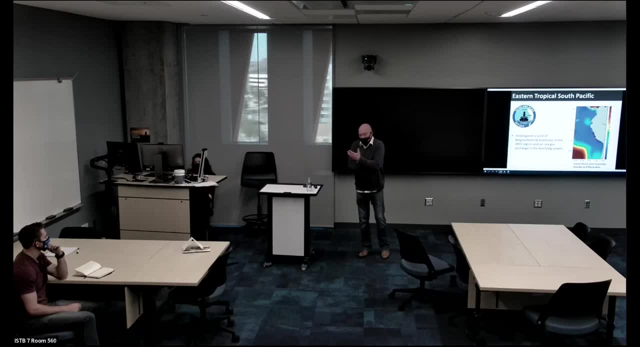 I'll work more with the biogeochemical modelers for that. But I really think we're going to start to see an increase, a very large increase, at some point And that's going to get out to the atmosphere. But we then need to think about feedbacks that we might see. 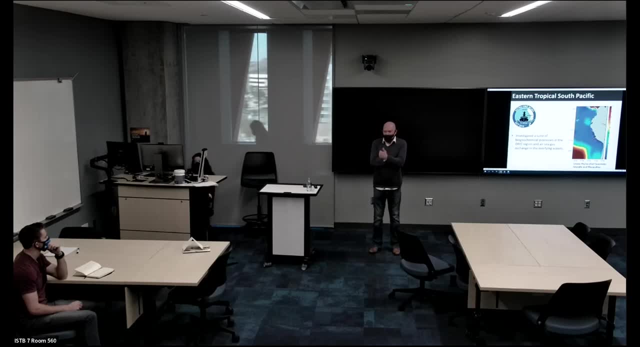 As I mentioned, on one hand, that could- That's going to be a positive feedback, So we might see more N2O in the atmosphere, warmer conditions, more stratification in the ocean, So even less sort of oxygen penetration and things like this, which could lead to even more N2O production. 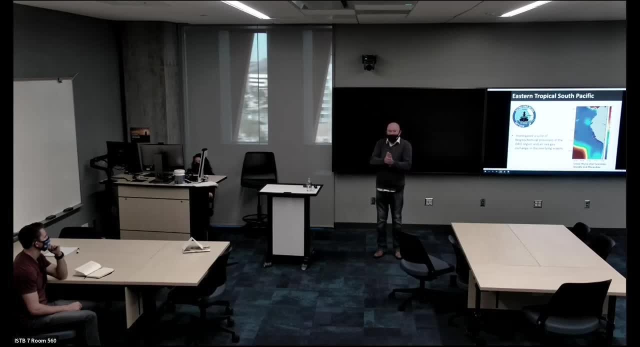 On the other hand, we could end up with a negative feedback system where we, Because of that stratification, we're getting less nutrients coming up to the surface, We're getting less primary production occurring, Less organic matter going down, So now we've got less oxygen being consumed. 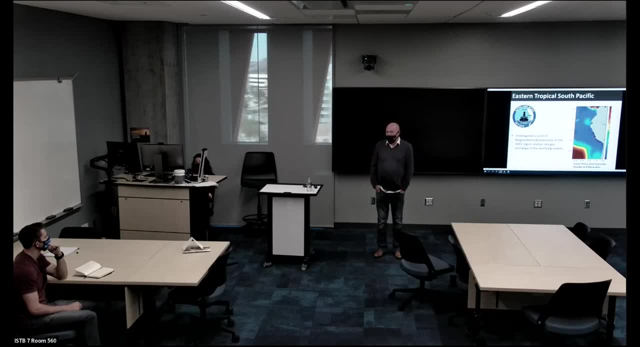 I think this is a very complex sort of thing to look at And it really needs some hardcore modeling techniques to be done. Peter, you have one On the topic of extrapolating forward, If you take your best guess of what an extreme situation of the increase of N2O production in the ocean could be. by whatever 2050, 2100, you could pick the time of that- which fraction of the greenhouse gases would actually be N2O rather than CO2, COCs, etc. So in other words, how big will the effect actually be? 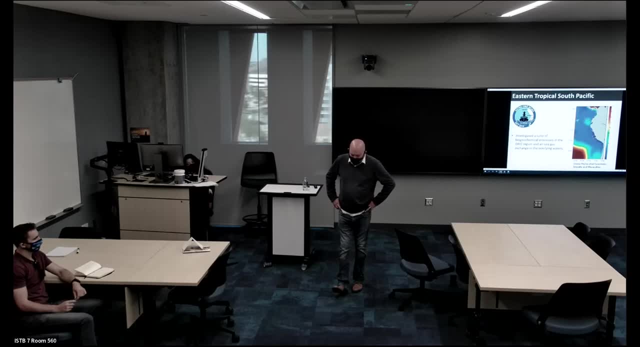 Is it a few percent? Is it shifting? We typically say two thirds or so is CO2.. And then we have methods, And then we have the main ones. So what could the envelope be in which N2O might reside in the future? 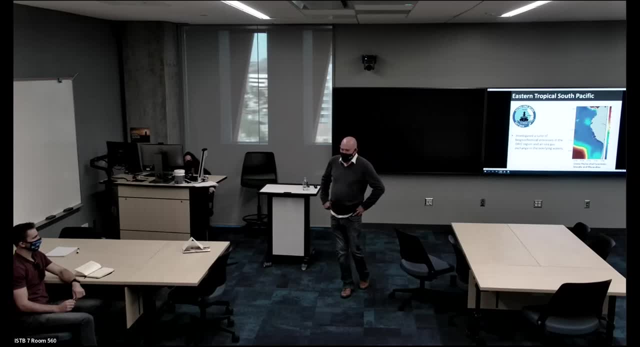 I'm not sure I'm going to commit to that. I'm just looking for some. I do understand how early it is in your research, But if you would say what is your best guess? Or you could even call it speculation, Just to get a sense. How much are we actually expecting? Maybe up towards maybe something like 5% to 10%. That's just thinking running back to the envelope on the fly there, Because I'd also have to think about how we're expecting methane to change as well. If methane is also increasing then it's going to keep dwarfing the impact of N2O. But N2O is not certainly the most important one out there, But it is having contributions And it's also. But it's going to be the number one ozone destroyer, for sure. 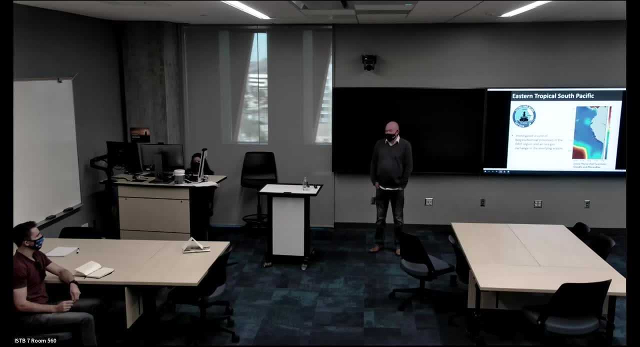 That would have been the next question, by the way. Yeah, Thanks. What if North Atlantic deep water formation slows down? How do changes in ocean circulation affect global marine N2O emissions? Yeah, If deep water formation slows down, we're going to have less option penetrating down depth and being transported. I mean it's one of the reasons why the Atlantic just doesn't have very low oxygen at the moment, Because we have that deep water formation starting off in that region. So certainly that could reduce- It's going to reduce- the supply of oxygen from surface waters down to intermediate depths, which is where a lot of the N2O is actually produced in the open ocean. 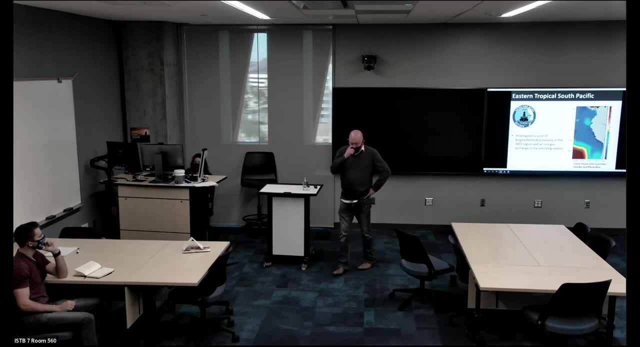 You can also think about it, as There's other interesting things as sea ice formation. We're getting much less sea ice formation And much more. Let me just see if I can quickly note this on my computer: We're getting much less sea ice being formed. And this is really slowing down the supply of oxygen. When sea ice is formed, you get brine rejections. This very salty, heavy water just extracts. It's taken out of the ice and it sinks down, taking oxygen down with it. 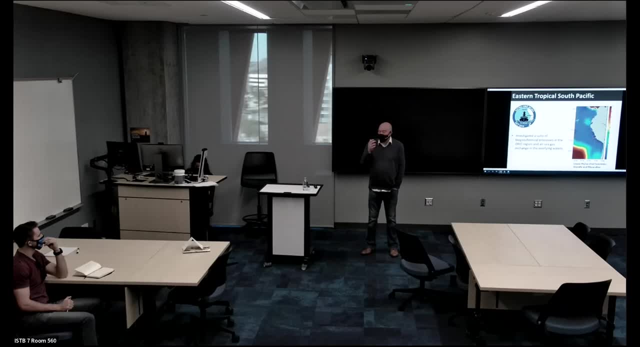 So that's. We're already seeing that happening in the Atlantic. We see it a lot in the Northeast Sub-Arctic Pacific. So there's a time series station there, Ocean Station Papa, where it worked a lot in the past And from the 50s they've been looking at oxygen concentrations. And they've been decreasing. It decreased by probably about 25% now at intermediate depths And that's going to speed up, Because what happens is over in the Sea of the Hoth. I can never really pronounce that Over in Russia you get a lot of sea ice being formed. 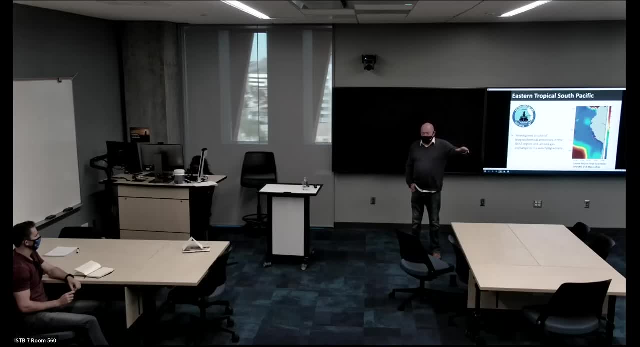 Well, typically we're getting much, much less sea ice being formed, So less oxygen, So less oxygen is getting down to those intermediate depth waters, into the intermediate depths, which then transit across the Pacific over towards the Northeast Sub-Arctic Pacific. 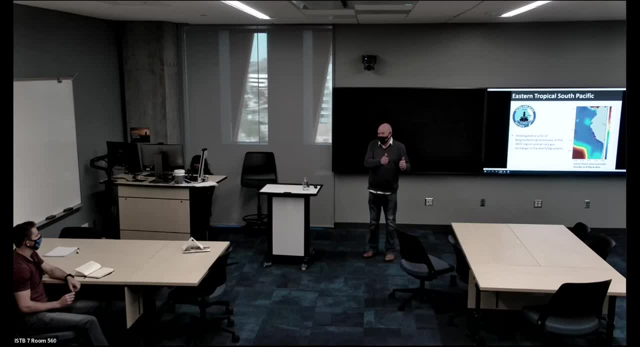 So we're getting much less oxygen being supplied, So we're just not starting off with as much oxygen as we typically would have. So just to clarify, when you're talking about sea ice formation in the Atlantic sector, you're probably looking at the area south of the silt of the Greenland, Iceland, Scotland silt. 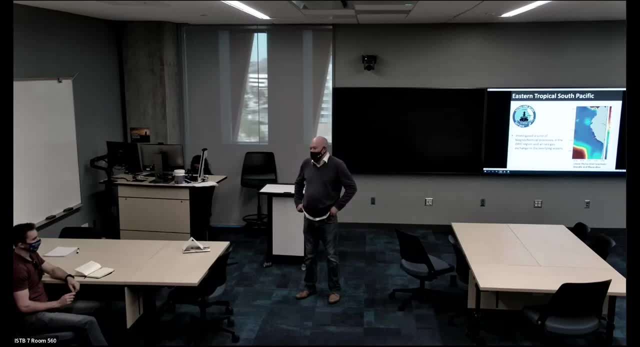 Yeah, And that's in the Arctic. Yeah, So you're probably going to have very little, very little, very little sea ice in the Atlantic, So it's going to be seen as more oxygen III. Yeah, That's a lot of positive feedbacks. Yes, But I think there are certainly at some point you're going to get to a negative feedback. Imagine if we get So think about it from another way. If we're getting less oxygen, we're getting more denitrification occurring eventually. 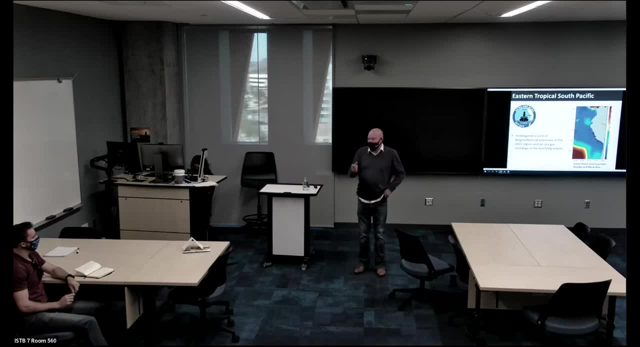 And so we're going to have maybe consuming N2. of dinitrogen gas being formed that leaves the ocean and just strips the ocean of bioavailable nitrogen. so now we just don't have any phytoplankton production occurring, but now we've got less co2 being taken up then from the atmosphere, um, or or by, you know, by- phytoplankton. 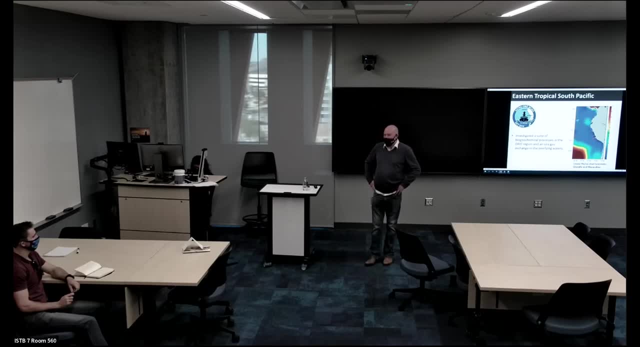 so there's, yeah, a lot going on there. that's why i say we shouldn't be drawing a line under this and saying where do we go? you know what's the what's the next thing? we want to work on it. so it could be busy for half a century, yeah. 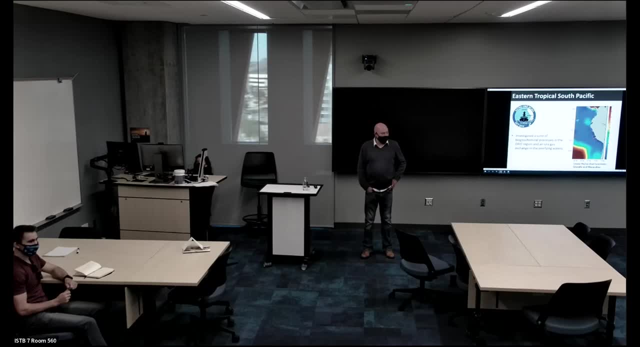 i don't have any other questions online um any others in the room. one final: yeah, so which fraction of the work that you're doing do you think you can do is for gliders, and at which fraction still needs conventional z-going? yeah, let's say, if most of my work is is nitrogen cycle, um. 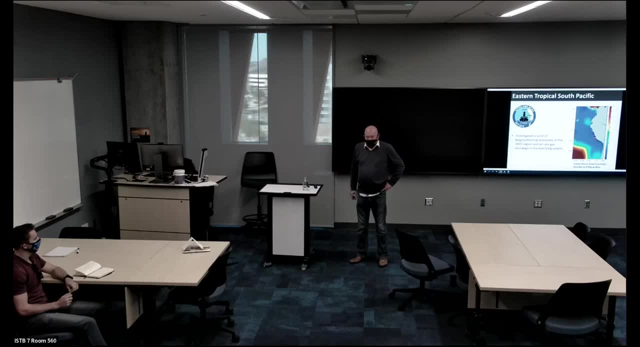 in terms of oxidative versus reductive nitrous oxide. we're just not there with gliders. um, there's, you know, we could use gas tension devices that we can put on the, on the instruments, to look at things like denitrification or signals and things like this, which i know. thank, 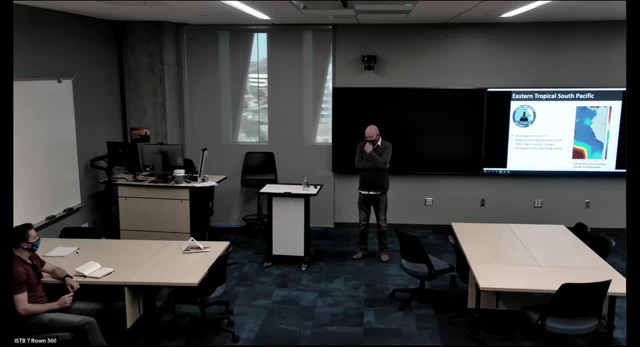 you. i believe you've worked with that quite a bit. um, there's certainly other automated things that know underwater submersible mass specs. i i think is a pretty cool idea. i even think that you could take the picaros and probably build an underwater pressure housing. and i've been thinking and